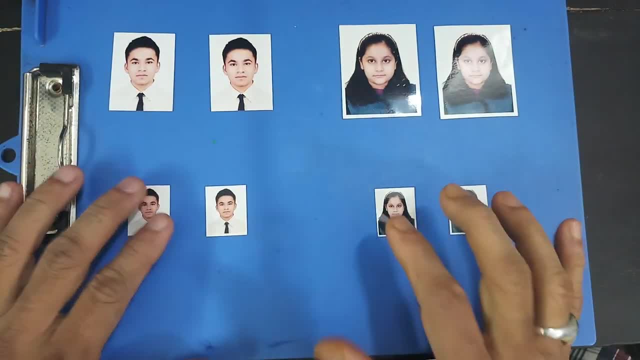 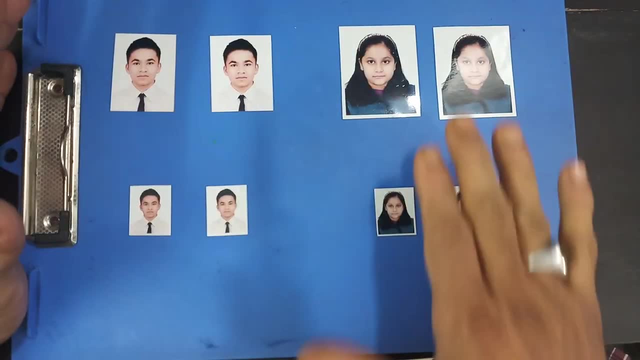 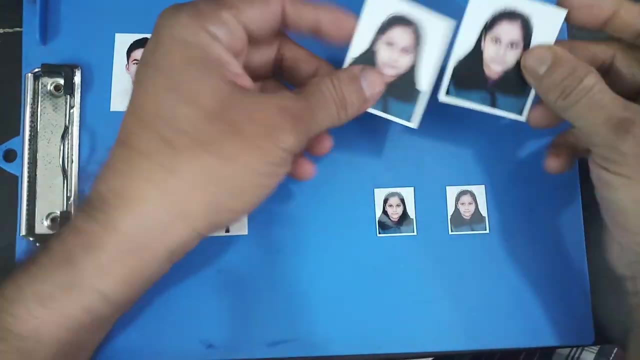 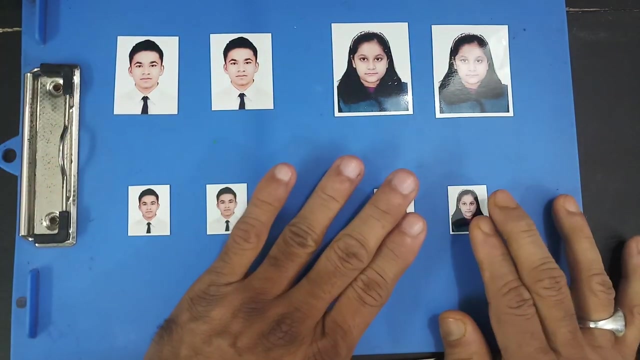 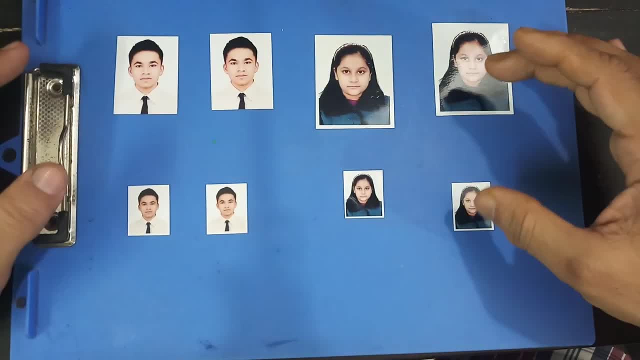 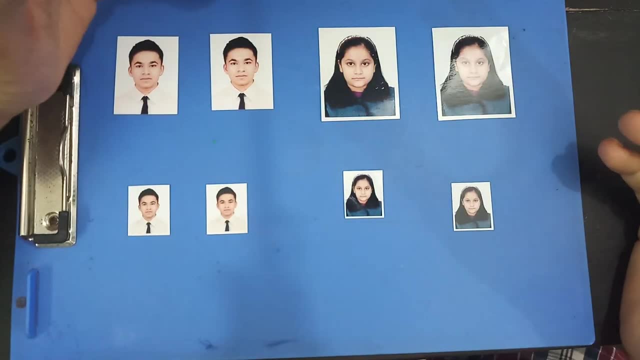 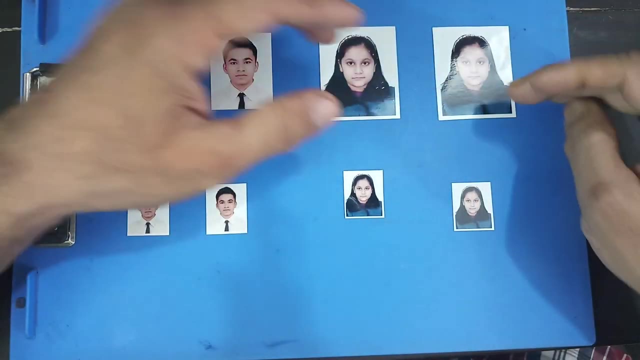 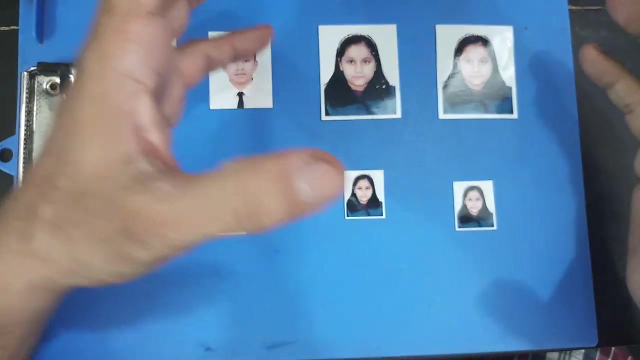 as a matter of fact, we can call all of them are similar, But congruent, are special type of similar thing that has all length, side, angle. they are equal to each other, Okay, but similar means that they are proportionally either small or big. So this photograph from this one is proportionally small, Or we can say that this photograph from this one is proportionally large. Okay, so these are. these are similar. 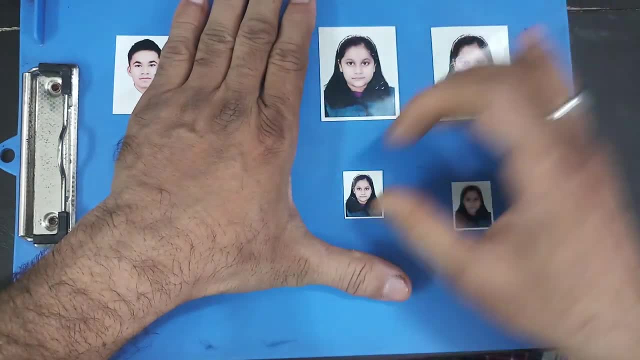 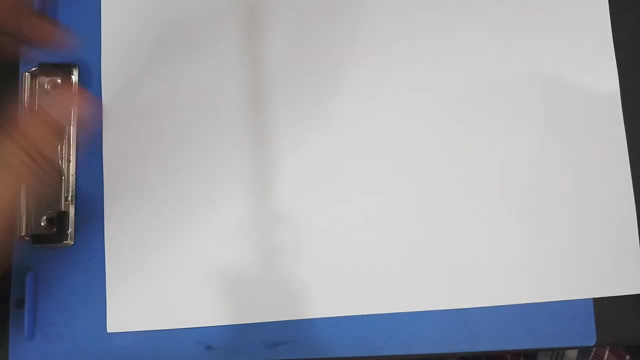 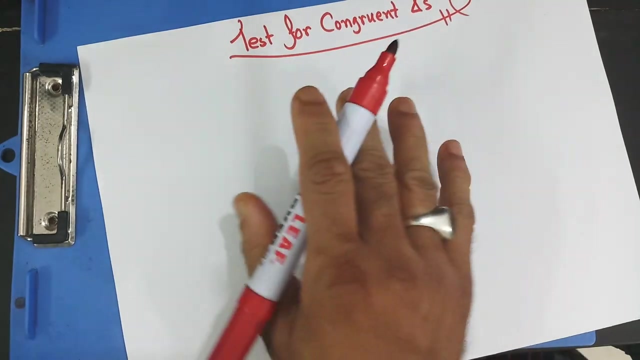 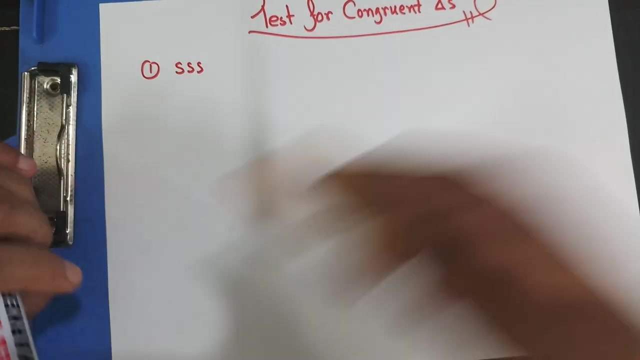 photographs, But especially these two are known as congruent. These two are congruent. Today, I'm going to talk about congruent triangles. Okay, Now let's say what are congruent triangles and what are the test of congruent triangles. Okay, Test of congruent triangles. we have four tests. One is known as SSS, And that actually means side side. 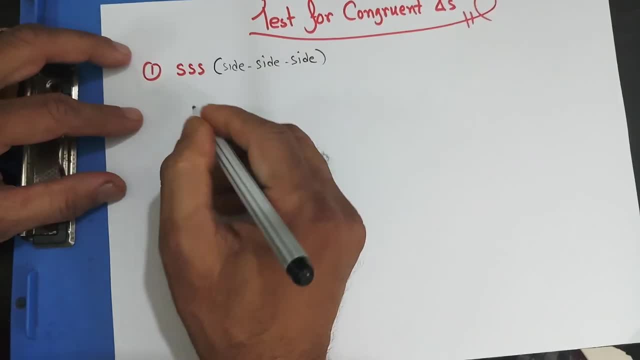 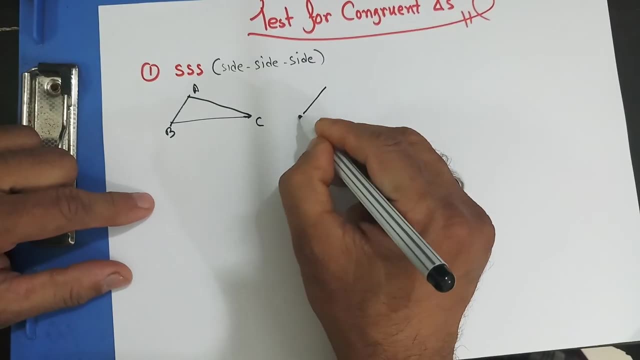 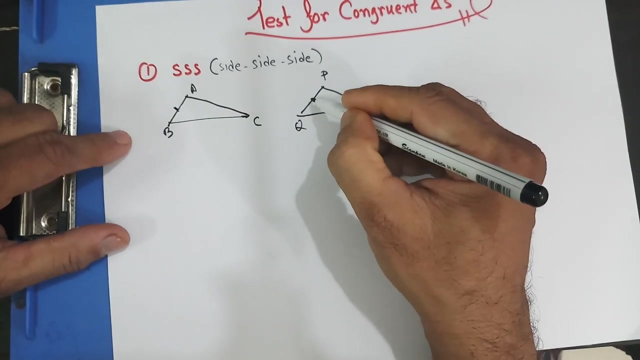 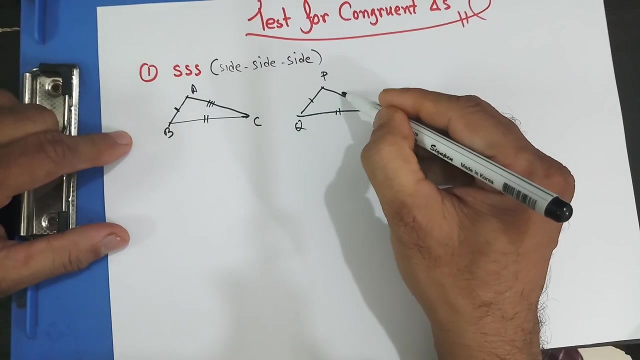 side. Okay, If I have a triangle, is such this one, ABC, And then I have another triangle, that PQR, And if it's given that AB equal to PQ and BC equal to QR and AC equal to PR, then these two triangles are congruent. 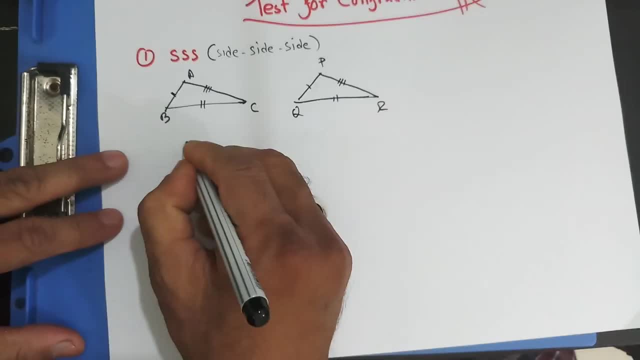 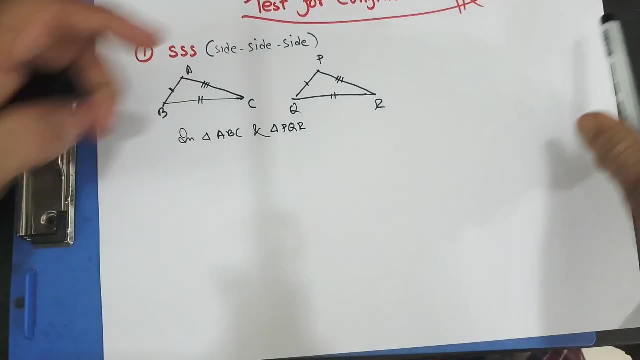 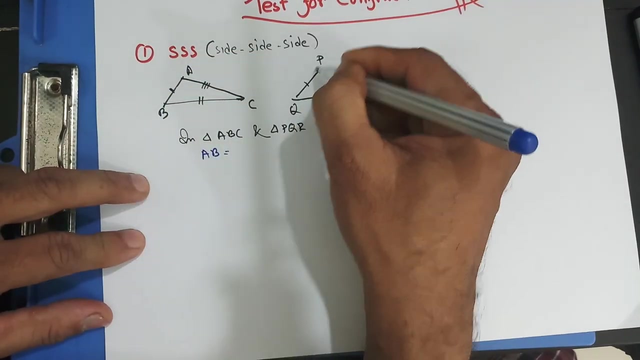 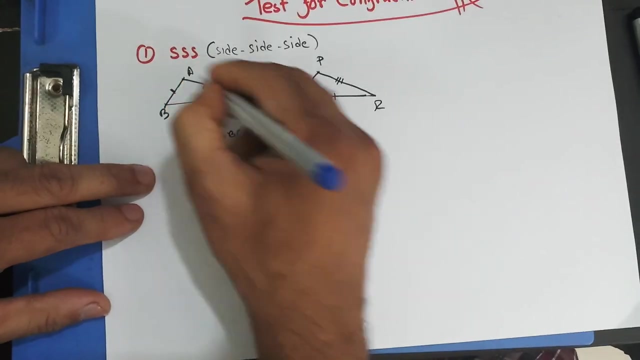 Okay, so what we're talking about? we are talking about in triangle ABC and triangle PQR. Okay, Then what happened? We have AB equal to AB, equal to PQ, then BC equal to QR and AC, or you can go counterclockwise: AB, BC, CR. 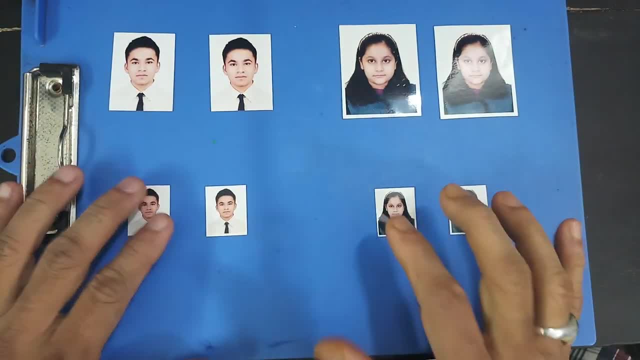 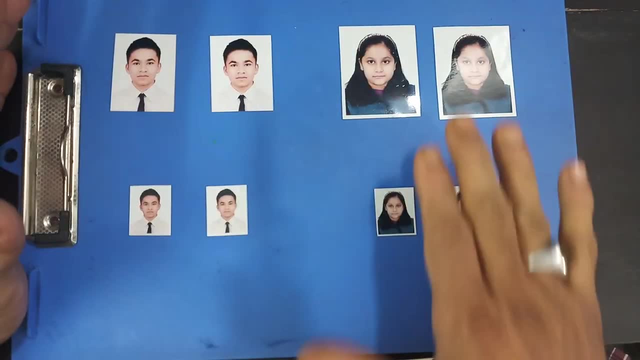 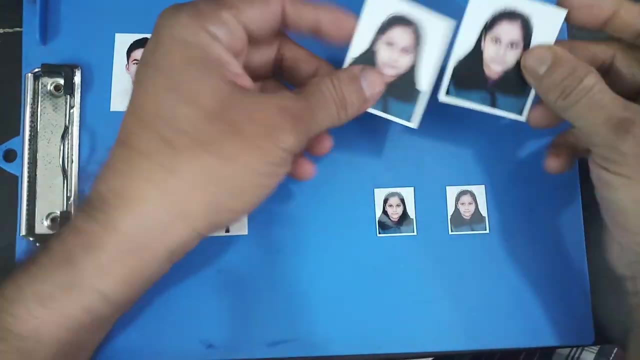 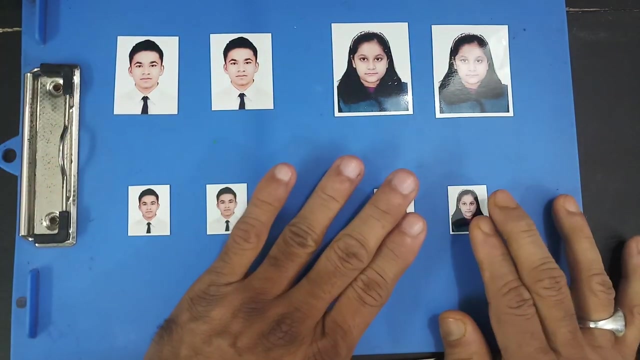 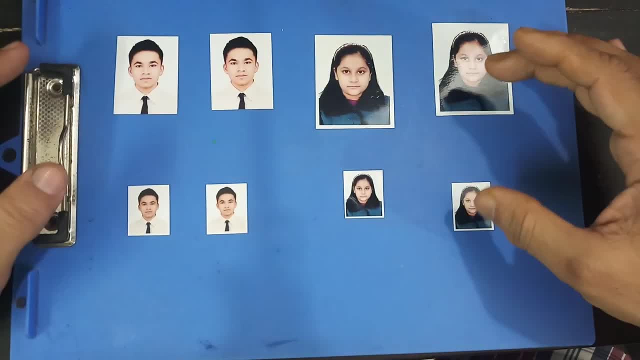 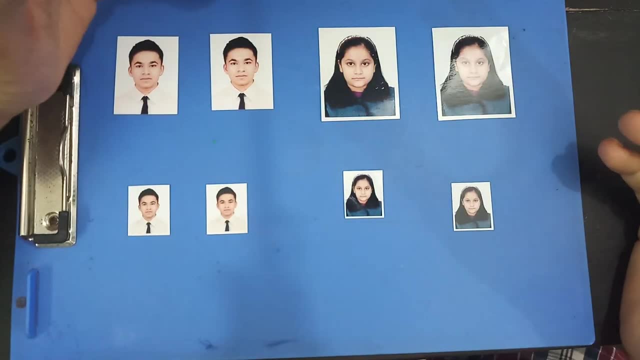 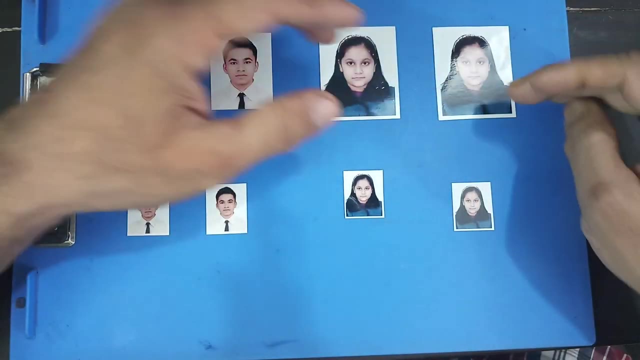 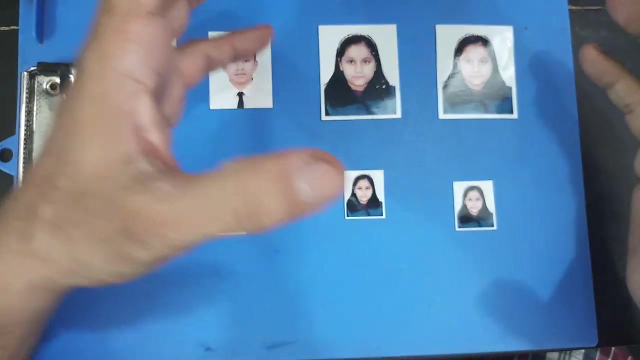 as a matter of fact, we can call all of them are similar, But congruent, are special type of similar thing that has all length, side, angle. they are equal to each other, Okay, but similar means that they are proportionally either small or big. So this photograph from this one is proportionally small, Or we can say that this photograph from this one is proportionally large. Okay, so these are. these are similar. 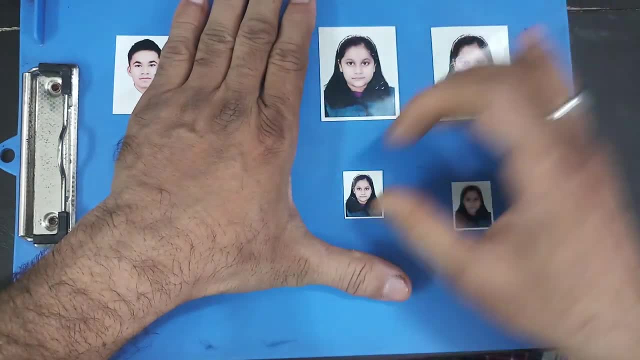 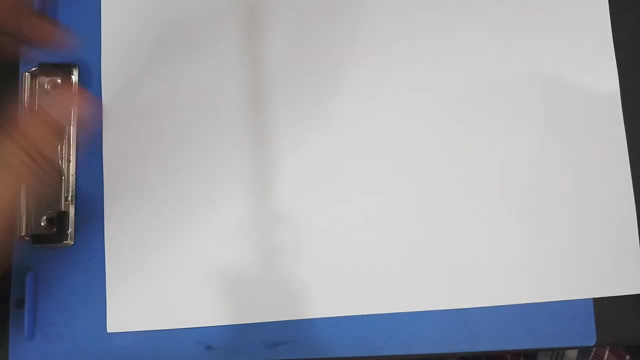 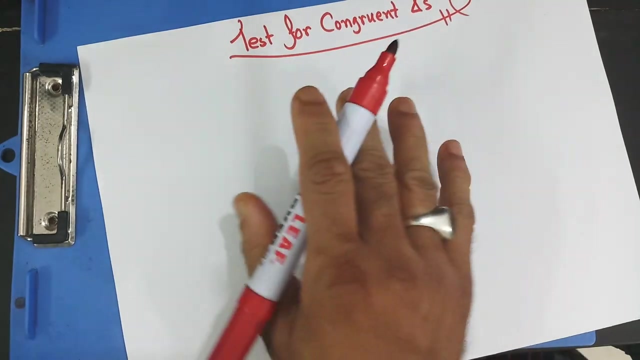 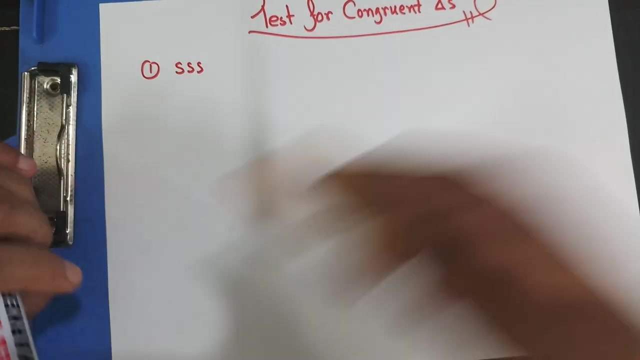 photographs, But especially these two are known as congruent. These two are congruent. Today, I'm going to talk about congruent triangles. Okay, Now let's say what are congruent triangles and what are the test of congruent triangles. Okay, Test of congruent triangles. we have four tests. One is known as SSS, And that actually means side side. 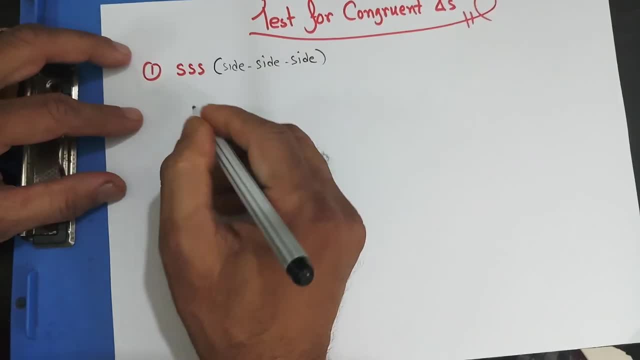 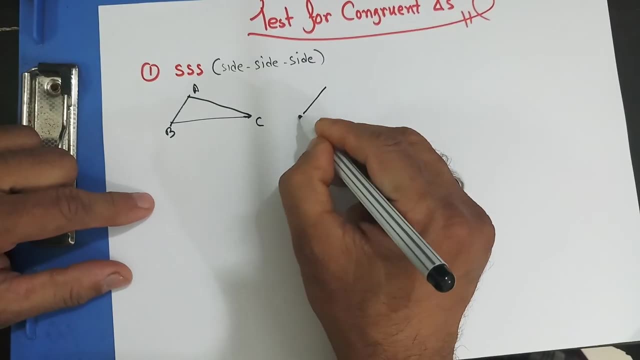 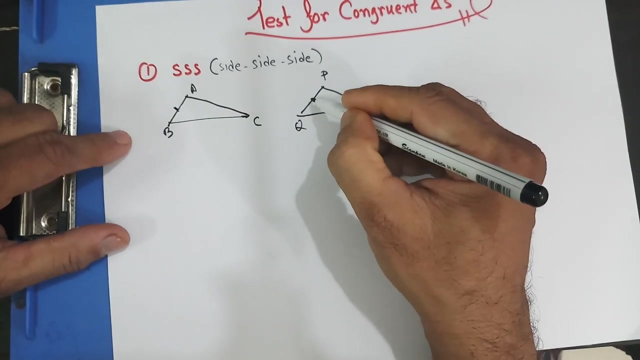 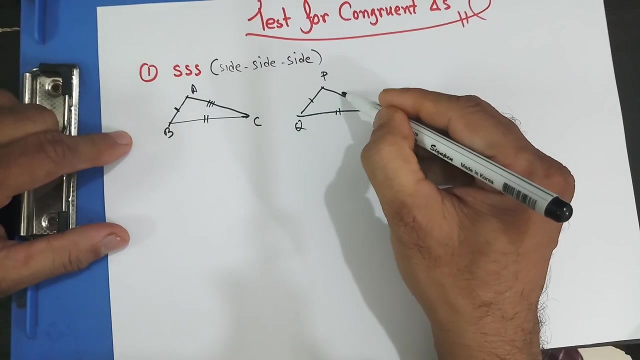 side. Okay, If I have a triangle, is such this one, ABC, And then I have another triangle, that PQR, And if it's given that AB equal to PQ and BC equal to QR and AC equal to PR, then these two triangles are congruent. 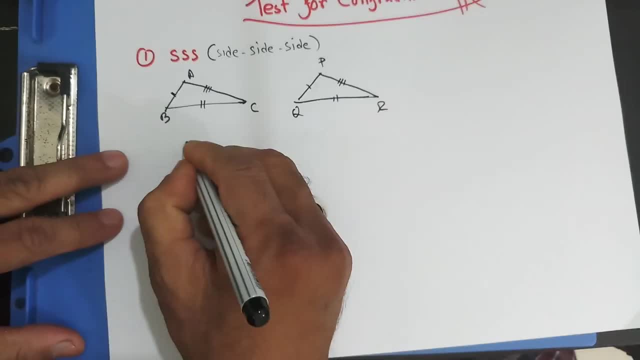 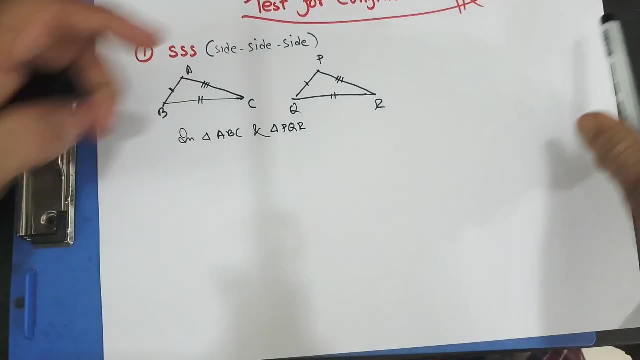 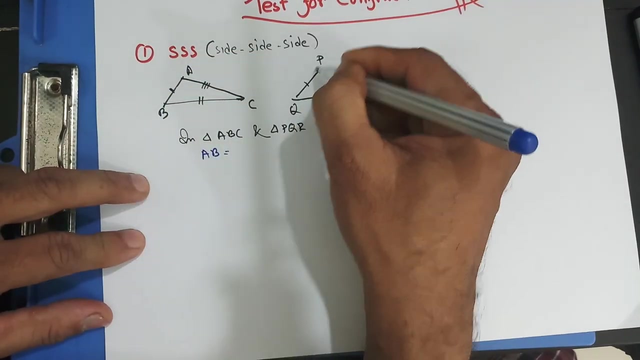 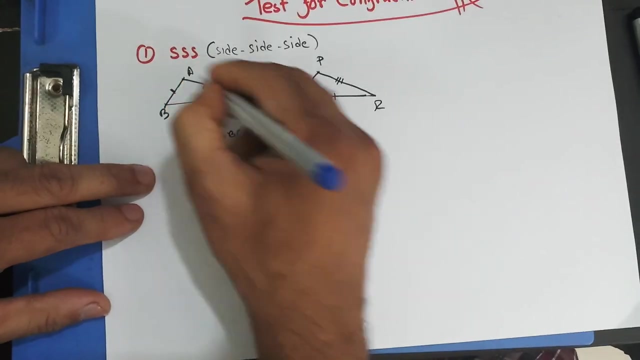 Okay, so what we're talking about? We are talking about in triangle ABC and triangle PQR. Okay, Then what happened? We have AB equal to AB, equal to PQ, then BC equal to QR and AC, or you can go counterclockwise: AB, BC, CR. 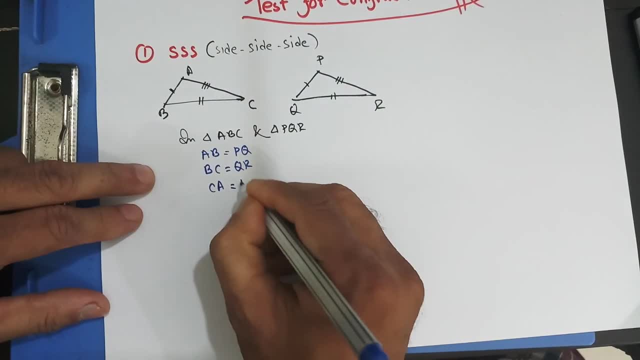 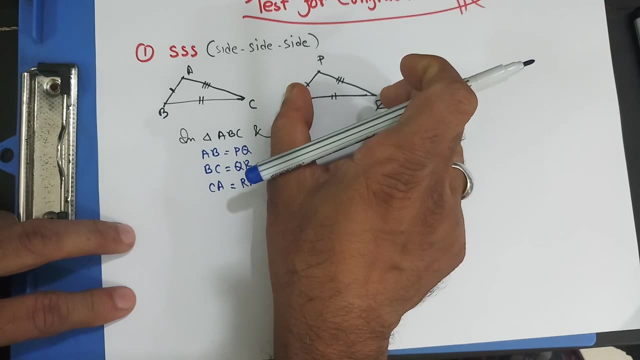 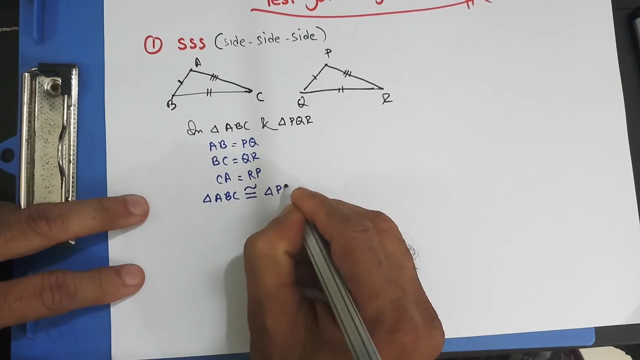 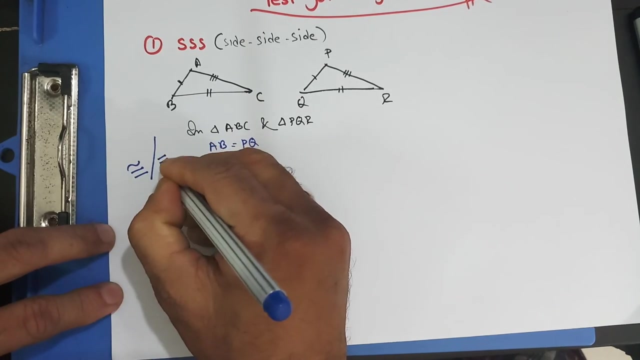 CA. then we have to go RP, RP. Okay, When three sides of a triangle equal to three sides of another triangle, then we can say: these two triangles are congruent. Okay, we can write down congruent like this: The symbol is like that congruent symbol is like this. Or sometimes we write down it like that: congruent, Okay, this is equivalent to, or we can write down it like that: congruent. 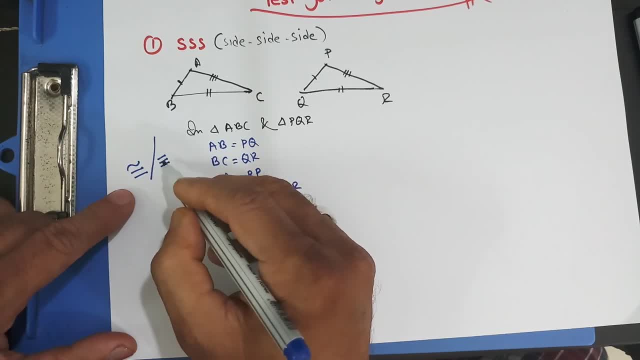 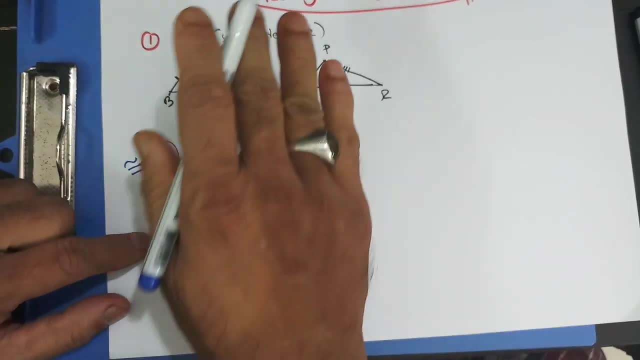 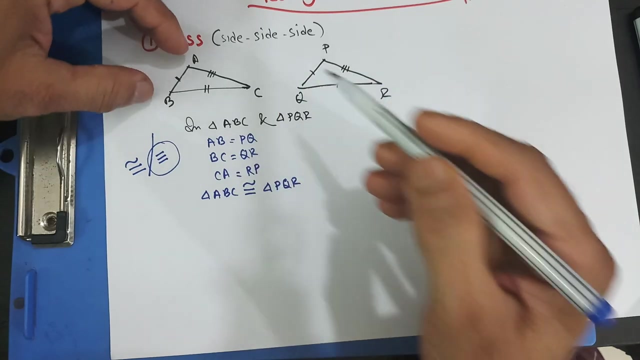 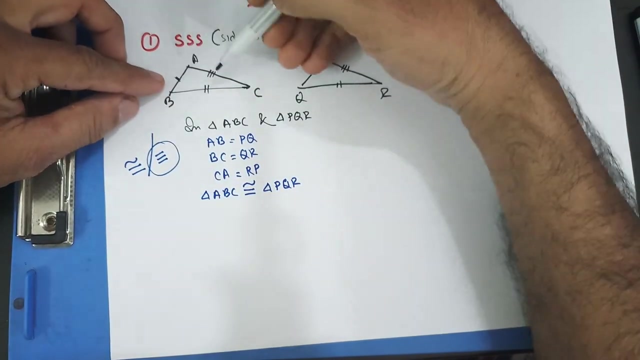 Okay. Then some of the teachers, some of the book, use this is for the congruent, this symbol for the congruent, and some use that: Okay, Most of the time I use this Okay, So this is congruent. This is one of the test of congruency for the triangle. But there you have noticed one thing: See that AB. length AB and length PQ. I wrote down: they are equal. See that one bar, this one bar. whenever you have seen in the geometry shapes that one bar and there is another bar. 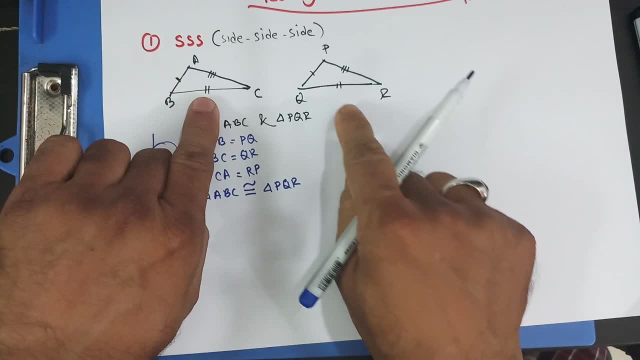 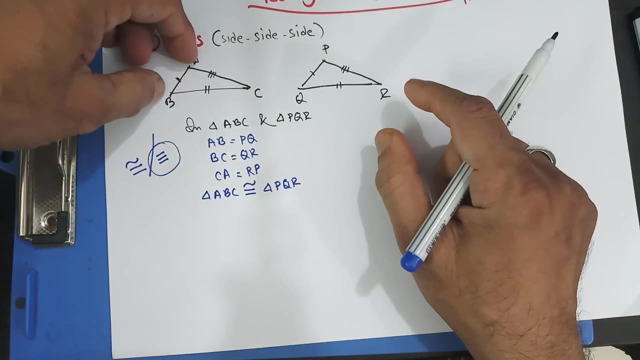 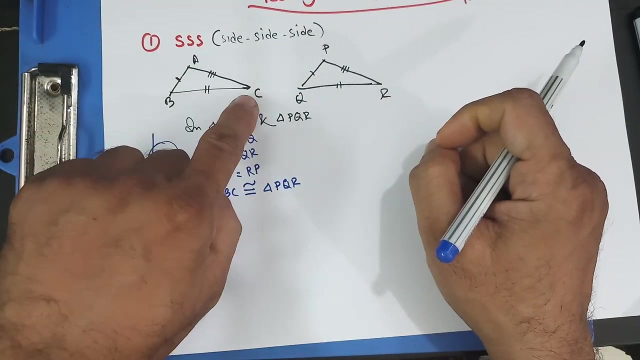 you can say that these two are equal, And over here two bars and over here two bars, So these two are equal. These two bars and these three bars are never equal. So this is a pattern that when you see one bar in the same shape, same problem, one bar in one place and another bar in another place, then you can say these two are equal. So AB equal to PQ, they have one bar, BC equal to QR, they have two bars. And CA equal to RP, they have three bars. Okay, so they are equal And you can write down. 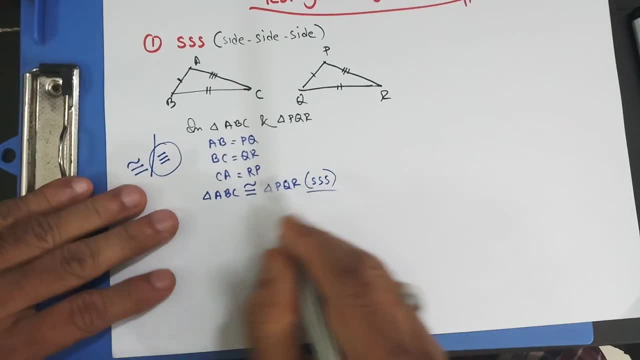 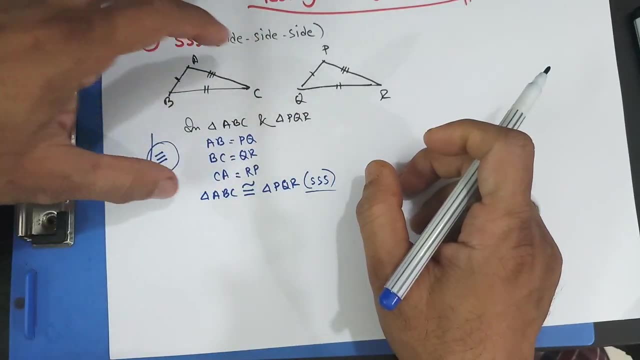 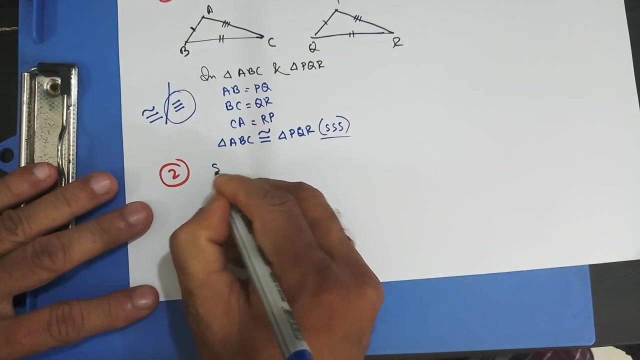 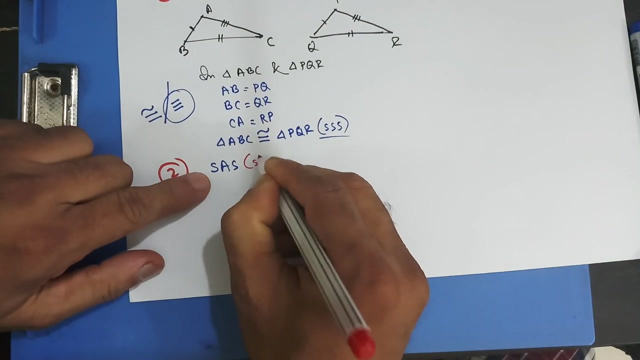 SSS. That's the test of congruency. After you write down two triangles are congruent, you always have to show the test of congruency. In this case it's SSS. Okay, Now, what is the next one? Next one is: I'm going to go for SAS. Okay, Now, as it is, I'm just going to write down that S means side- You already have done that Side- And A for angle, And then that is side. Okay, 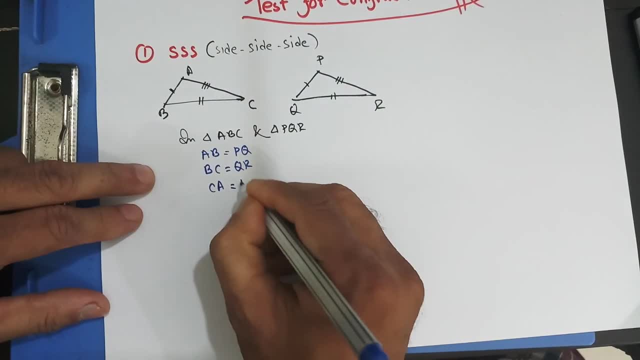 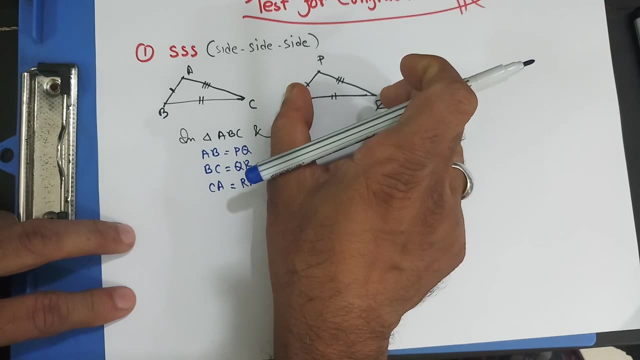 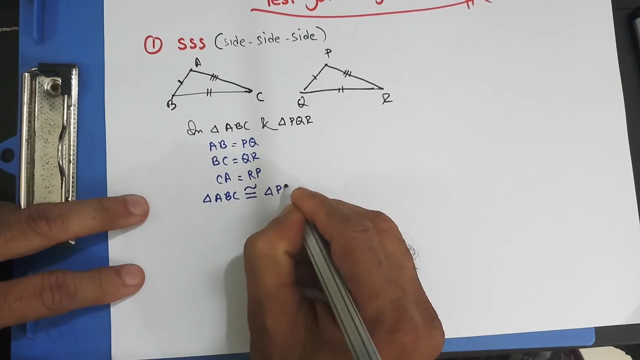 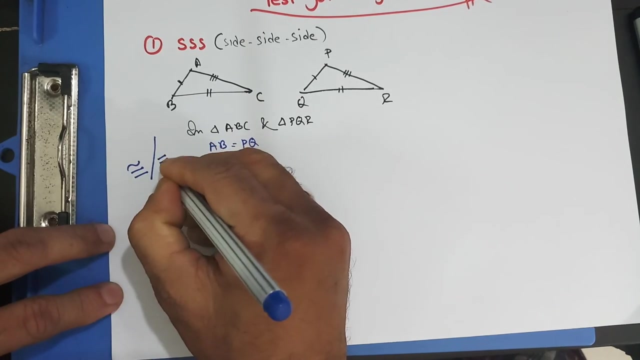 CA. then we have to go RP, RP. Okay, When three sides of a triangle equal to three sides of another triangle, then we can say: these two triangles are congruent. Okay, we can write down congruent like this: The symbol is like that congruent symbol is like this. Or sometimes we write down it like that: congruent, Okay, this is equivalent to, or we can write down it like that: congruent. 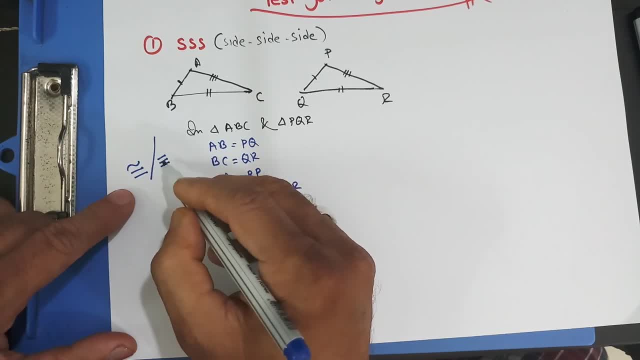 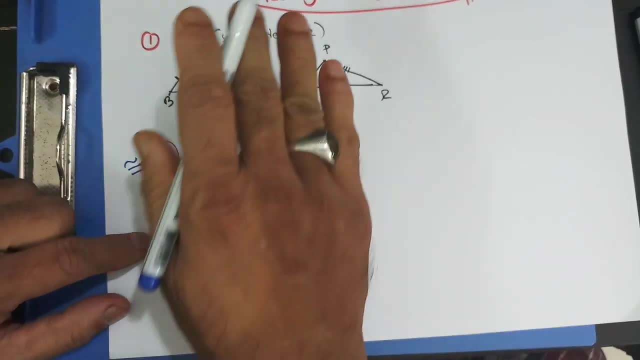 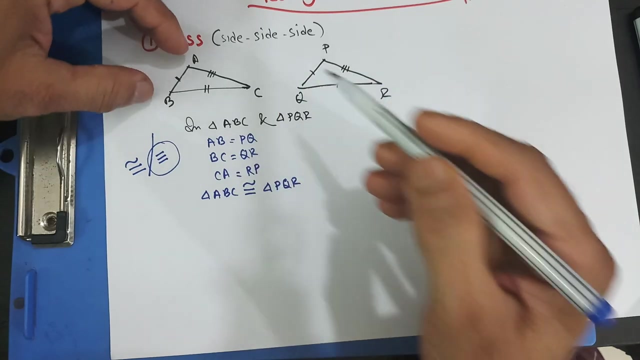 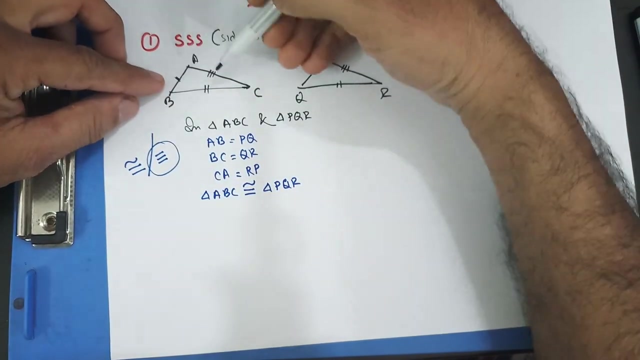 Okay. Then some of the teachers, some of the book, use this is for the congruent, this symbol for the congruent, and some use that: Okay, Most of the time I use this Okay, So this is congruent. This is one of the test of congruency for the triangle. But there you have noticed one thing: See that AB. length AB and length PQ. I wrote down: they are equal. See that one bar, this one bar. whenever you have seen in the geometry shapes that one bar and there is another bar. 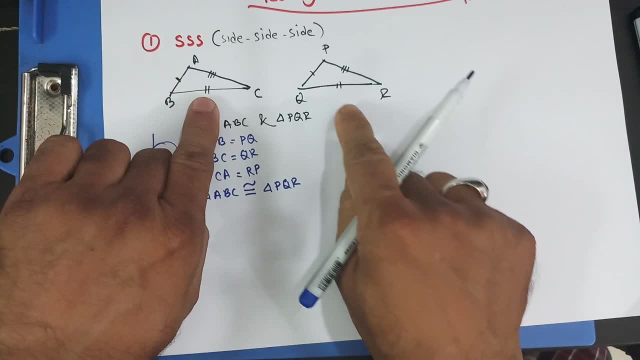 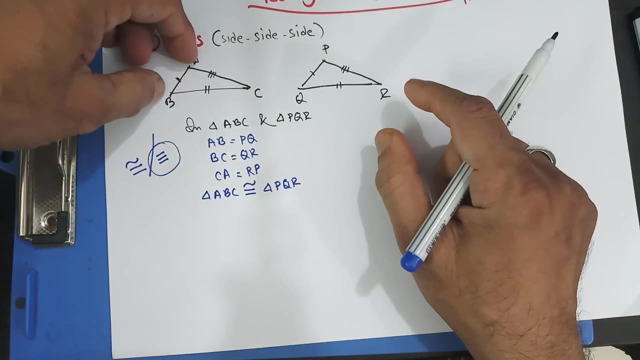 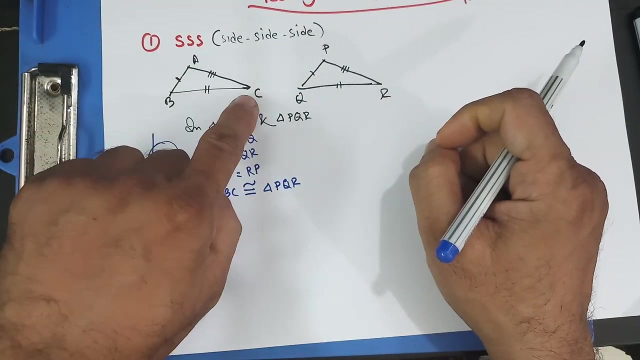 you can say that these two are equal, And over here two bars and over here two bars, So these two are equal. These two bars and these three bars are never equal. So this is a pattern that when you see one bar in the same shape, same problem, one bar in one place and another bar in another place, then you can say these two are equal. So AB equal to PQ, they have one bar, BC equal to QR, they have two bars. And CA equal to RP, they have three bars. Okay, so they are equal And you can write down. 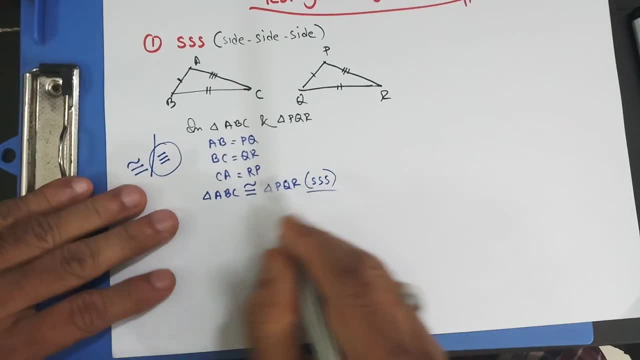 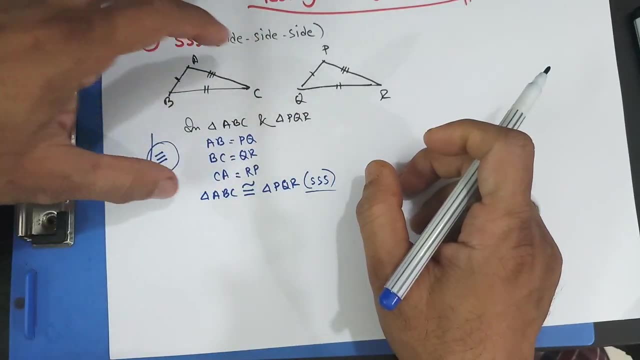 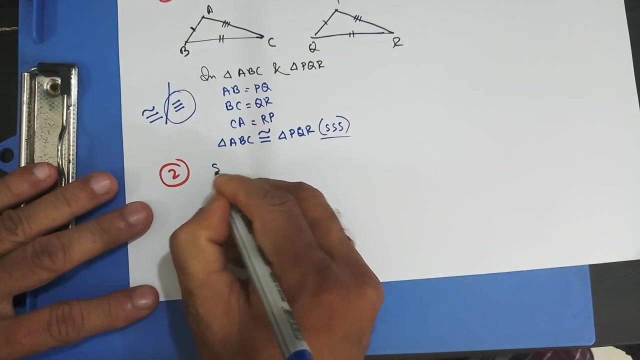 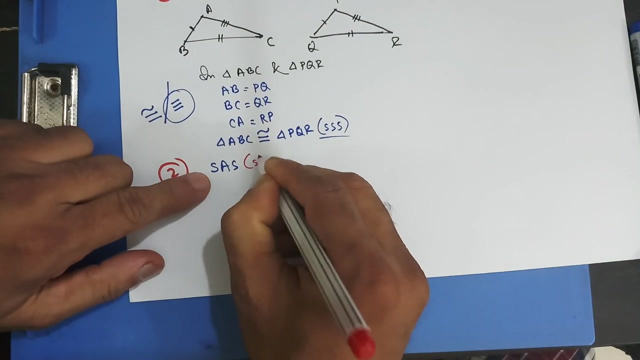 SSS. That's the test of congruency. After you write down two triangles are congruent, you always have to show the test of congruency. In this case it's SSS. Okay, Now, what is the next one? Next one is: I'm going to go for SAS. Okay, Now, as it is, I'm just going to write down that S means side- You already have done that Side- And A for angle, And then that is side. Okay, 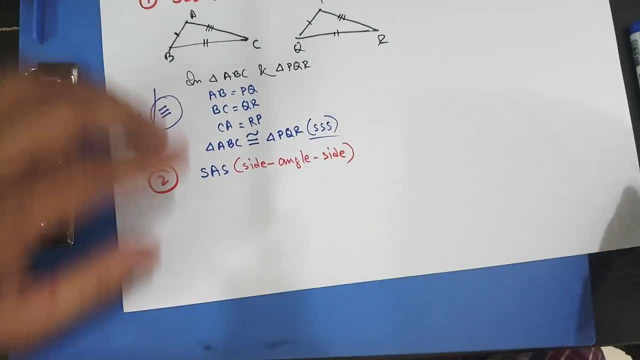 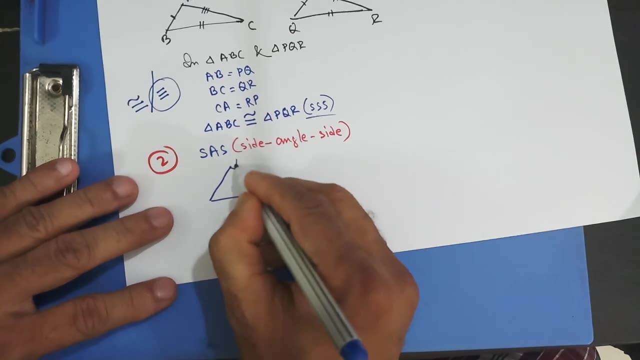 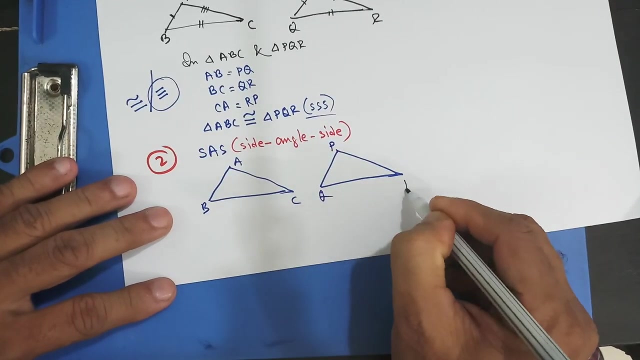 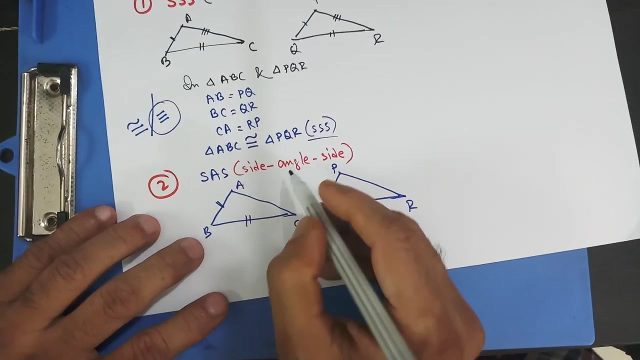 Okay, Now, this angle is little special angle. Okay, I'm coming to that in a second. So draw these two triangles: Triangle ABC and triangle same triangle. I'm going to put PQR. Okay, Two sides. So let's say this side equal to this side, This side equal to this side, And this angle is in between two sides, So we can say this one. 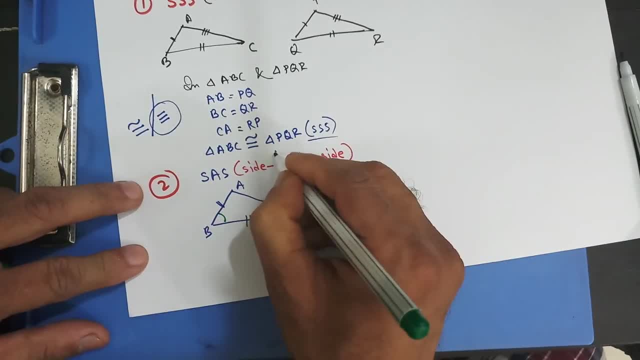 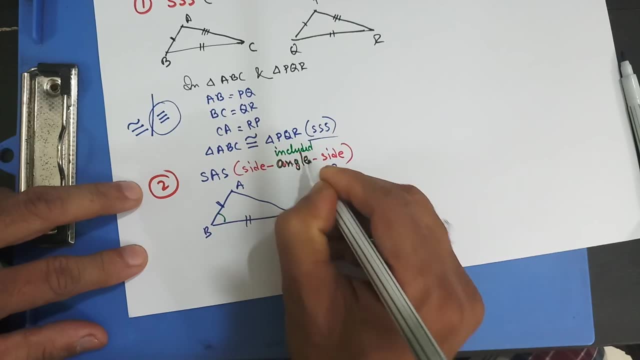 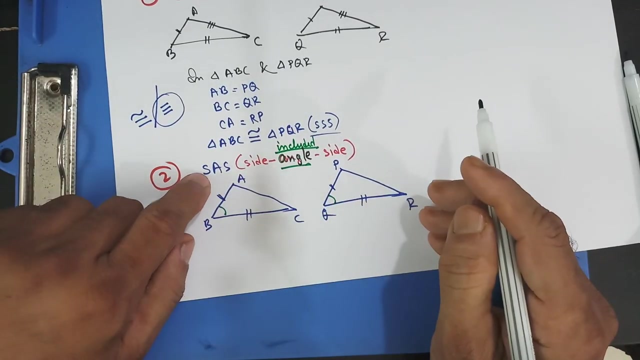 one, this, it has to be equal to that. okay, and we write down included angle. okay, included means in between this two given side included angle. we are not going to say side angle side, we're going to say side included angle side. so this side equal to this side, this side equal to this side, and in 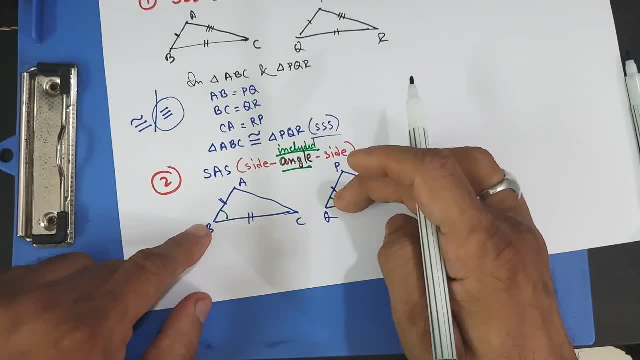 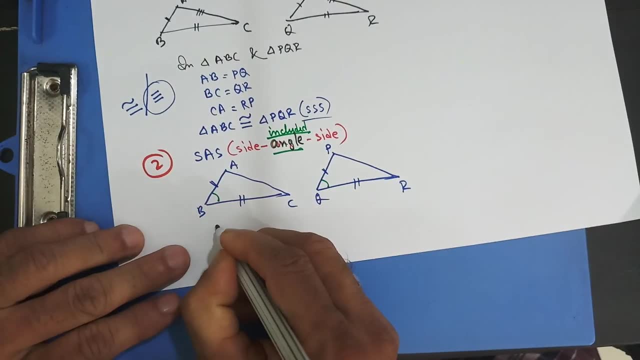 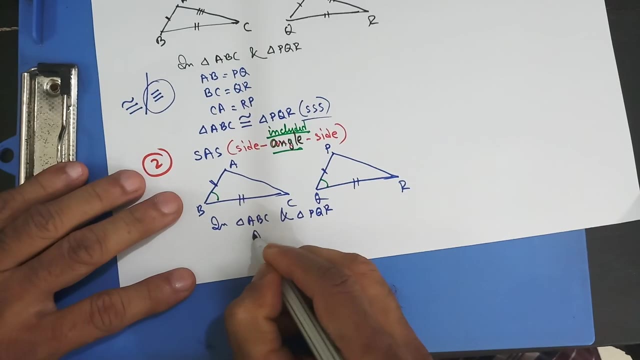 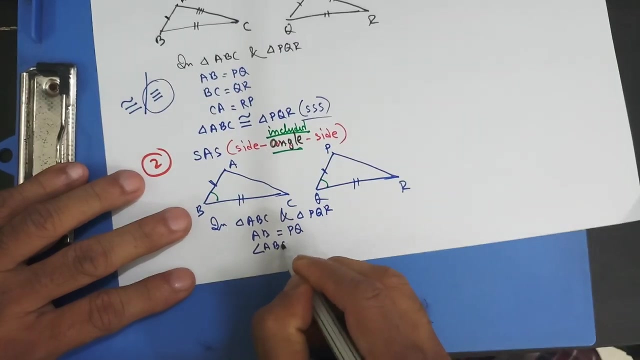 between these two sides. the angle i have, they are equal. okay, when i have any condition like that, then these two triangles are congruent. so let me write down that in triangles, in triangle a b c and triangle p q r, i have a b equal to p q. then you can write down angle a b c equal to angle p q r. 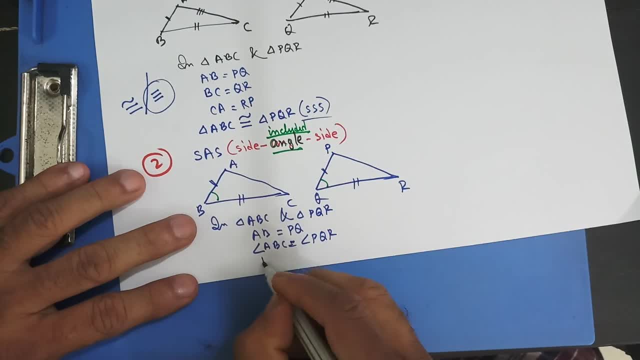 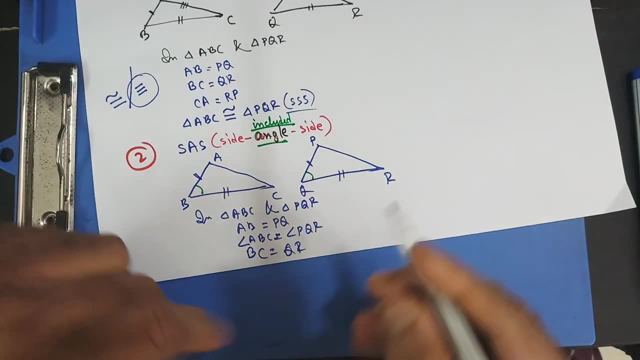 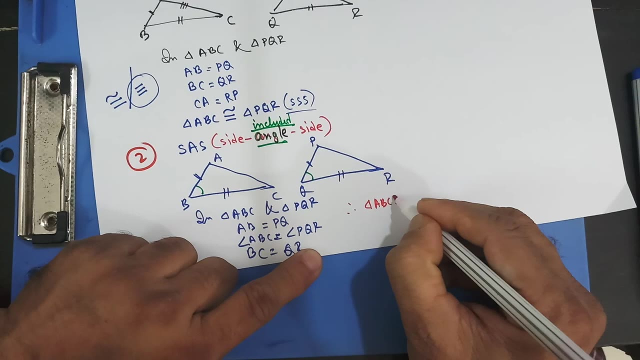 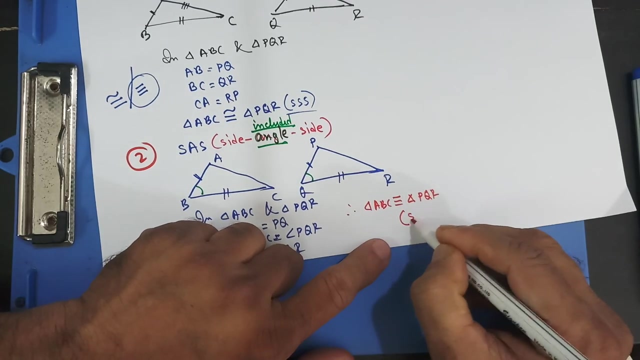 angle p, q r and b c equal to q r. therefore, we can write down down. therefore, we can write down: triangle ABC is congruent to- I have used this sign right right now I'm gonna use this- and both of them are equal. triangle PQR. and what is the test of congruency? side included, angle side or SAS? okay now. 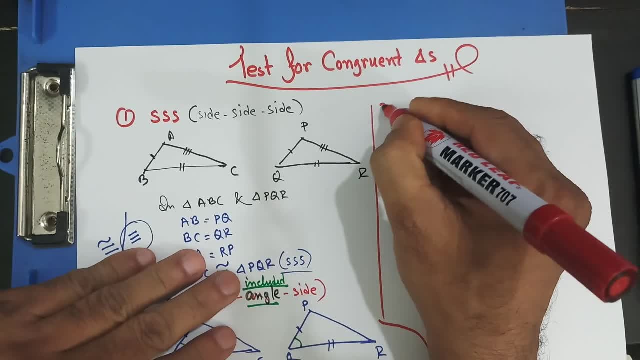 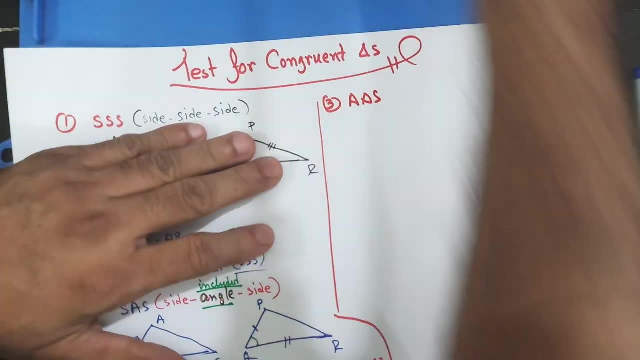 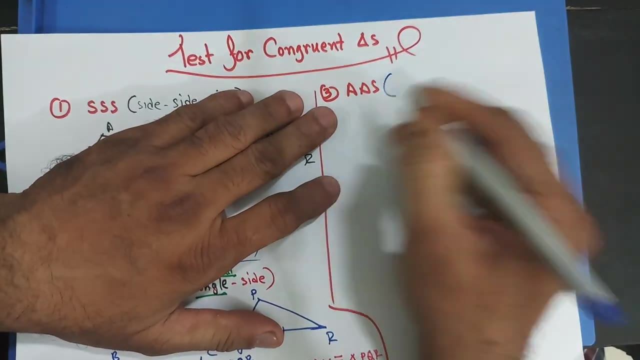 test of congruency number three: okay, and then this one is gonna be a, a yes, okay. whenever I write down on the board for the first time, student started to laugh and a smile and you, you can tell why. okay, but let me. let me write on this. 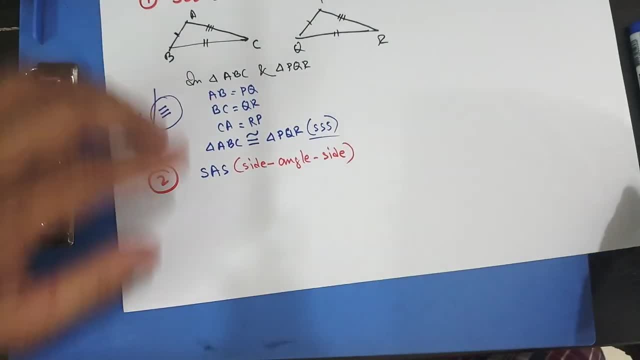 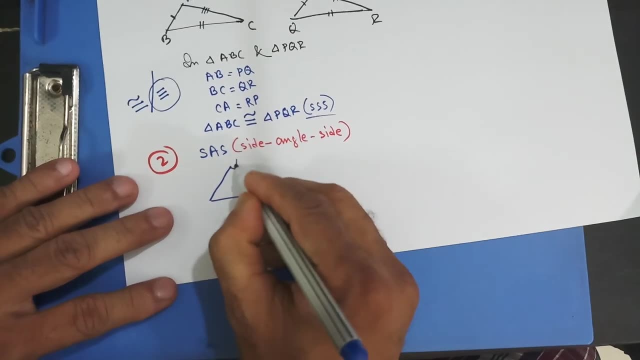 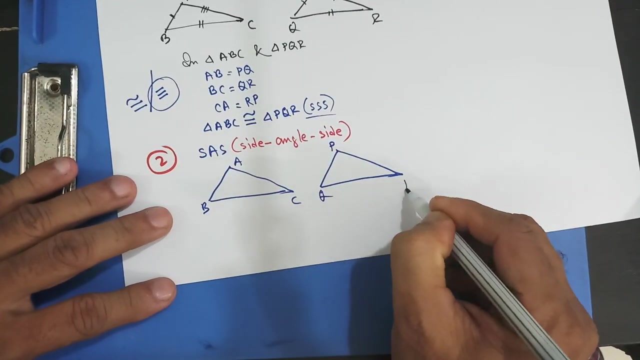 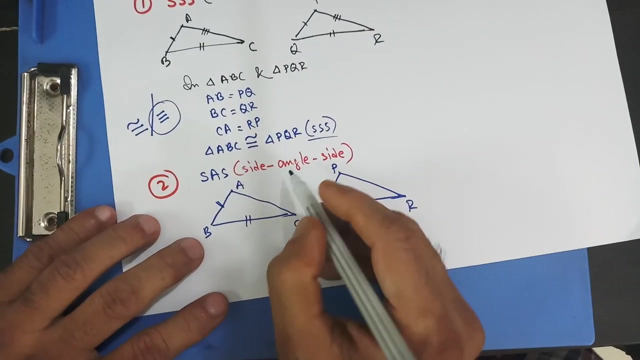 Okay, Now, this angle is little special angle. Okay, I'm coming to that in a second. So draw these two triangles: Triangle ABC and triangle same triangle. I'm going to put PQR- Okay, Two sides. So let's say this side equal to this side, This side equal to this side, And this angle is in between two sides. So we can say: 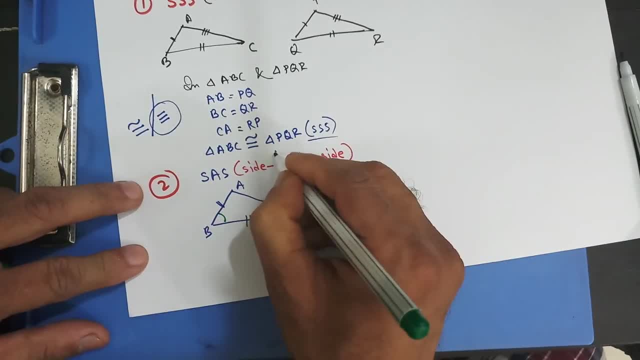 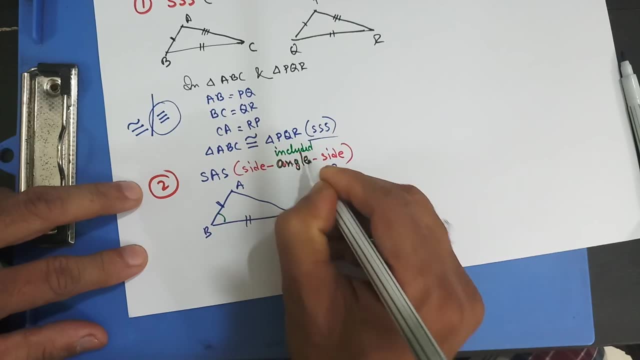 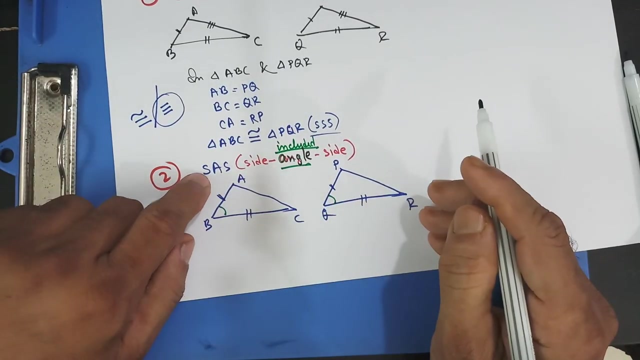 one, this, it has to be equal to that. okay, and we write down included angle. okay, included means in between this two given side included angle. we are not going to say side angle side, we're going to say side included angle side. so this side equal to this side, this side equal to this side, and in 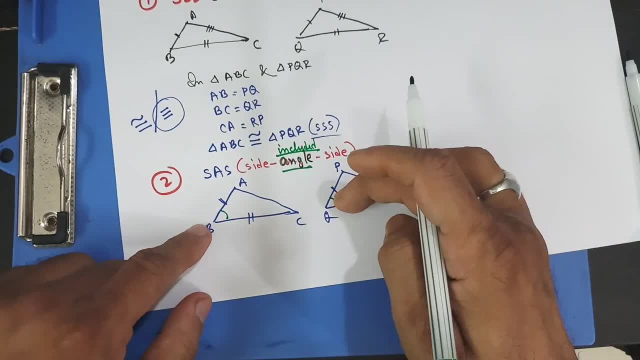 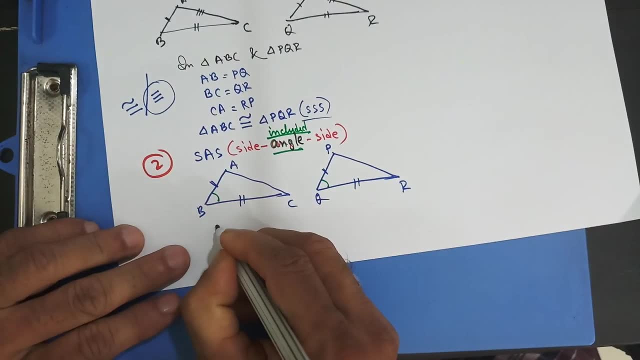 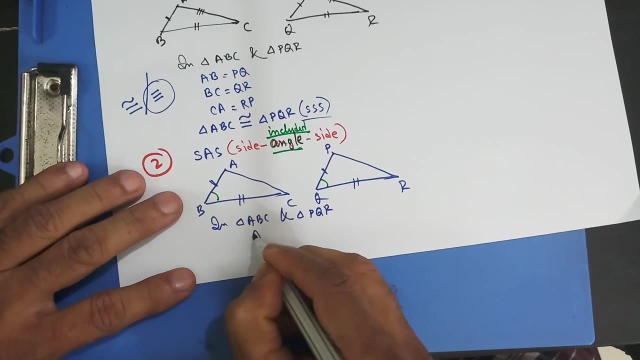 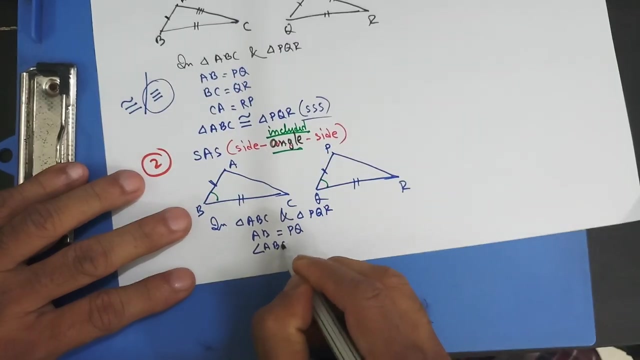 between these two sides. the angle i have, they are equal. okay, when i have any condition like that, then these two triangles are congruent. so let me write down that in triangles, in triangle a b c and triangle p q r, i have a b equal to p q. then you can write down angle a b c equal to angle p q r. 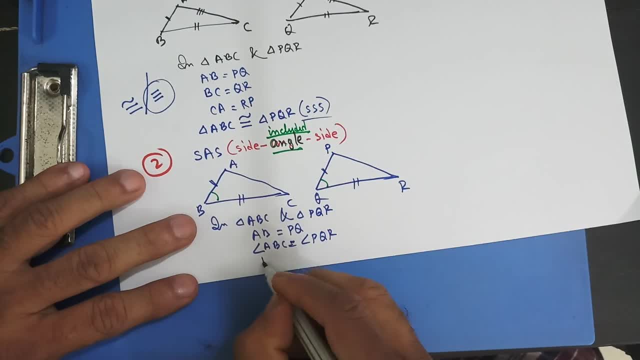 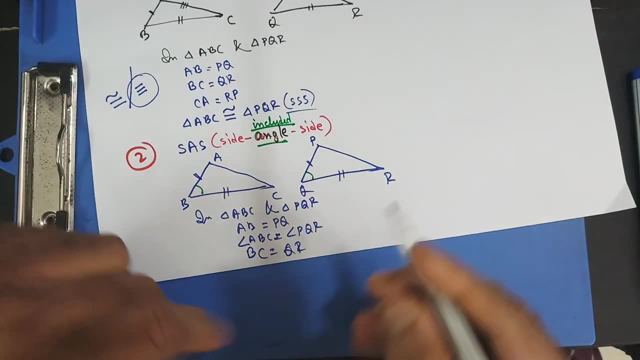 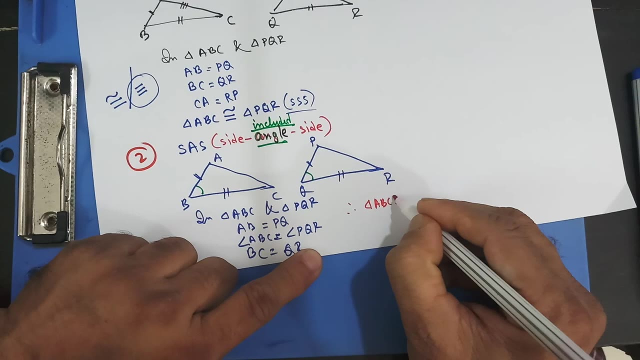 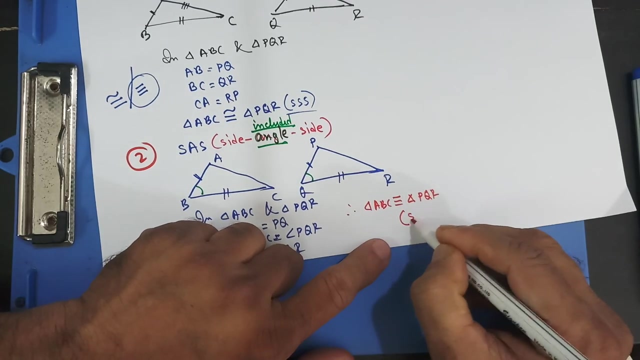 angle p, q r and b c equal to q r. therefore, we can write down down. therefore, we can write down: triangle ABC is congruent to- I have used this sign right right now I'm gonna use this- and both of them are equal. triangle PQR. and what is the test of congruency? side included, angle side or SAS? okay now. 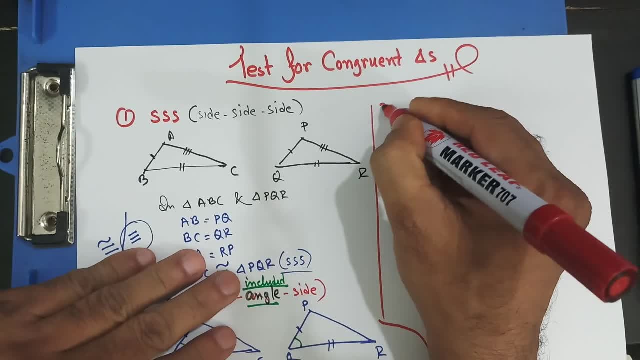 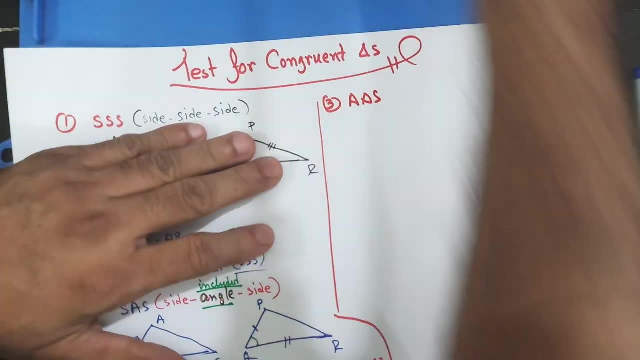 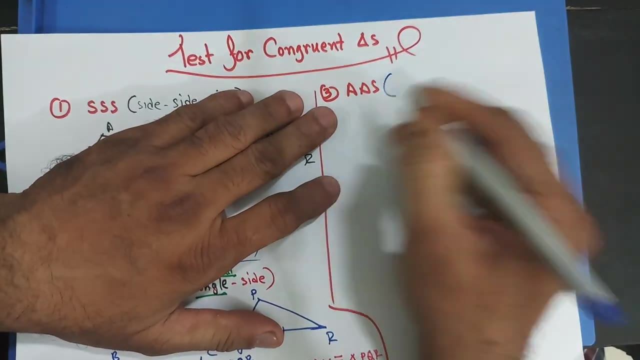 test of congruency number three: okay, and then this one is gonna be a, a yes, okay. whenever I write down on the board for the first time, student started to laugh and a smile and you, you can tell why. okay, but let me. let me write on this. 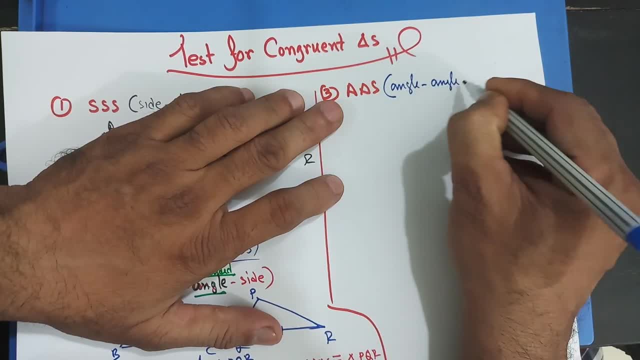 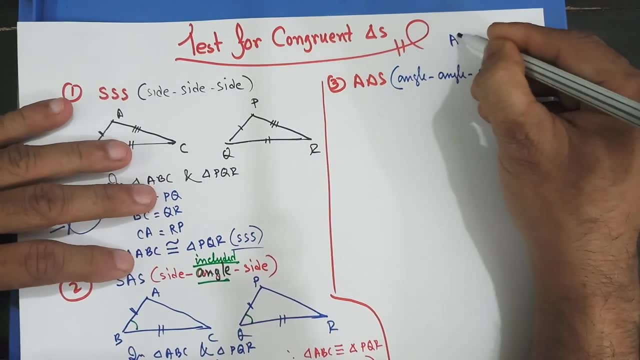 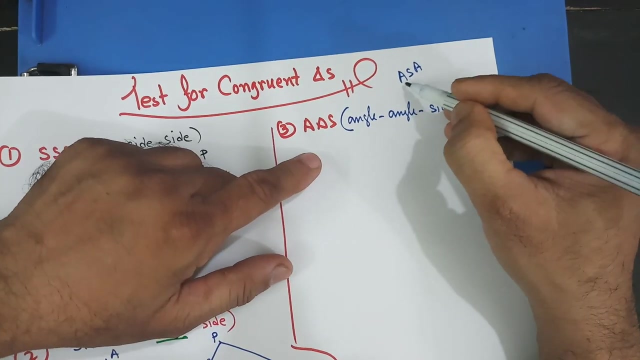 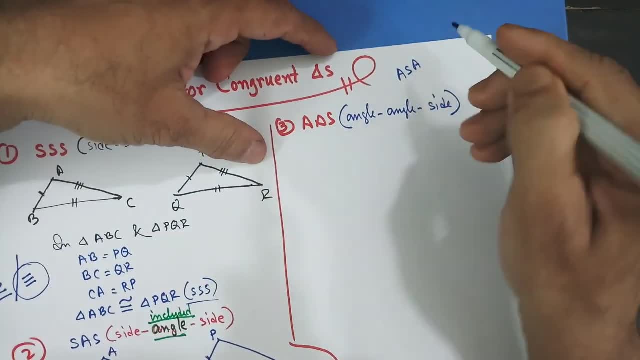 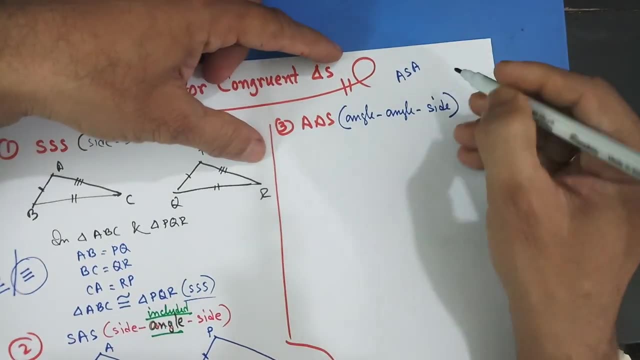 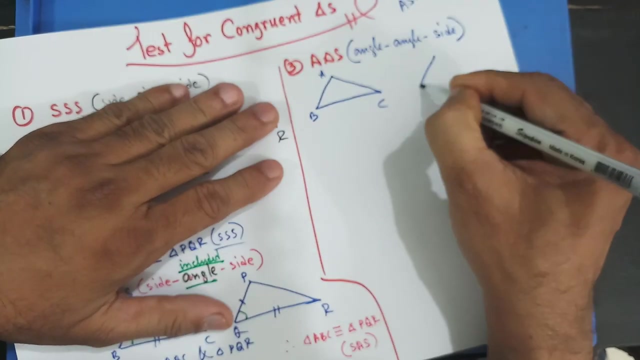 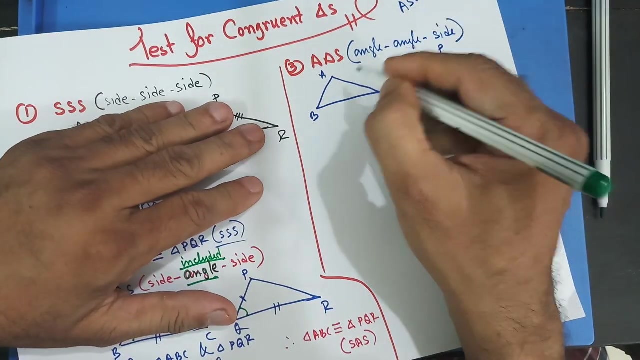 that side, corresponding side, but this is not the truth. okay, it should be corresponding side, but not included angle. if it's another side, it should be okay for congruency test. okay, let me give you this, this diagram first, then I'll explain. if I have ABC and over here I have PQR, okay, so over here, this angle a and this: 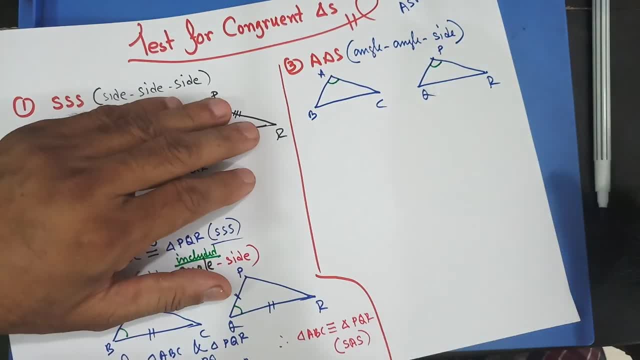 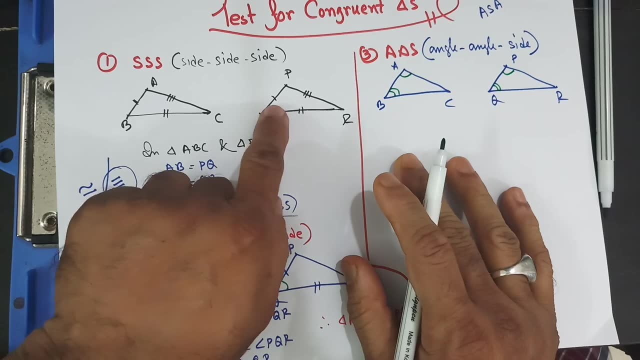 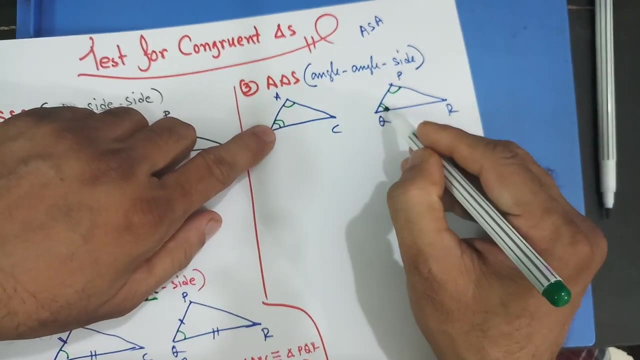 angle P, they are equal. and then I'm gonna use this: B equal to Q, same as one bar equal to one bar side over here for angle one arc length, one arc length, they are equal. and when I have two arc length, two arc lengths, these two are equal. so 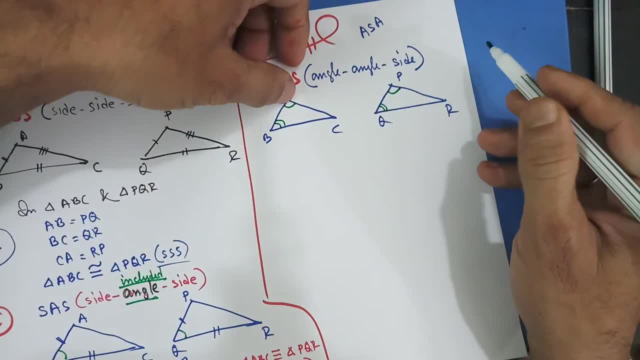 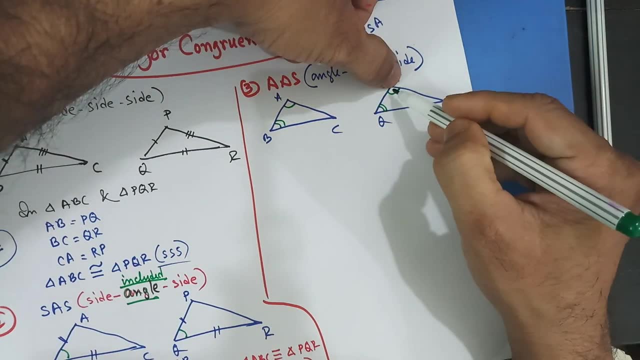 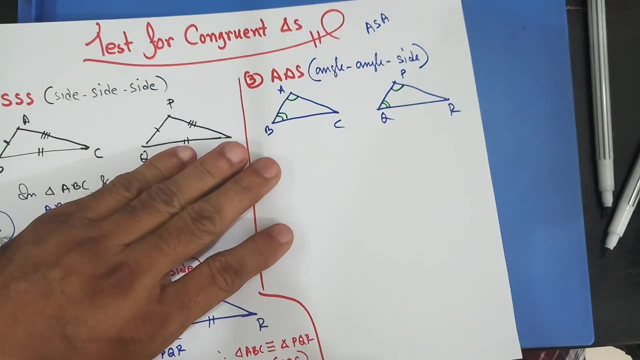 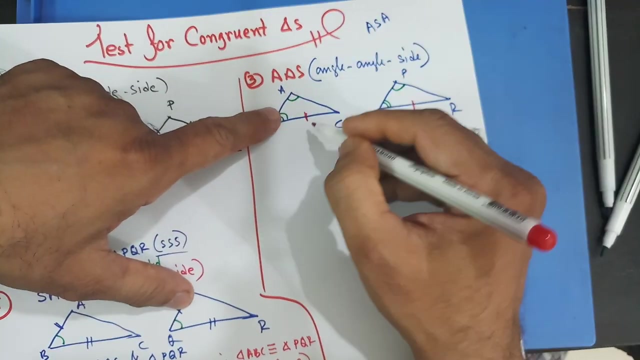 these two arc length and one arc length angle are never equal. in the same problem, same math, same diagram, if you have one arc length and another angle have one arc length. so these two are equal and two arc lengths, two arc lengths, they are equal. okay, now let's say I'm gonna say this side equal to this side given. okay, it has to be. 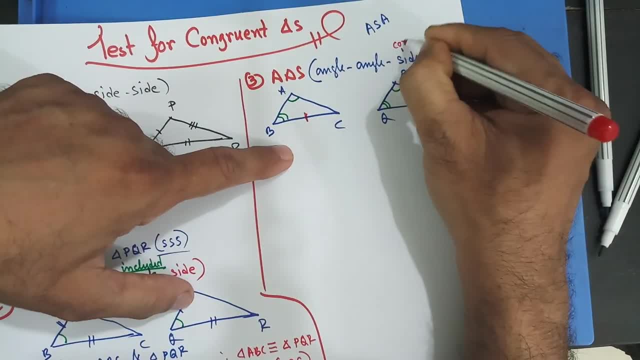 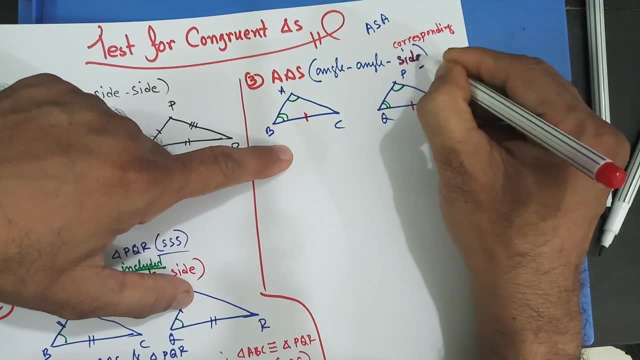 corresponding side. angle and arc length. start withipp. end of this cross prefix shape: okay, angle, corresponding side, not included angle. if it's included angle, it's gonna: okay, okay, but corresponding side. so in this case we're gonna say angle, angle and corresponding side. now, if i put: 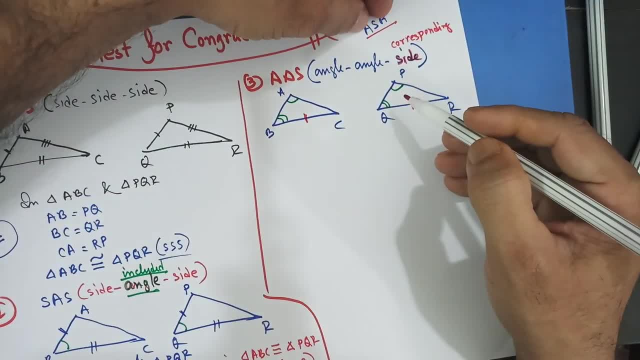 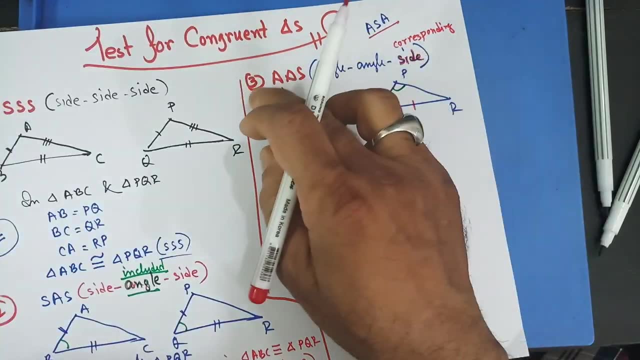 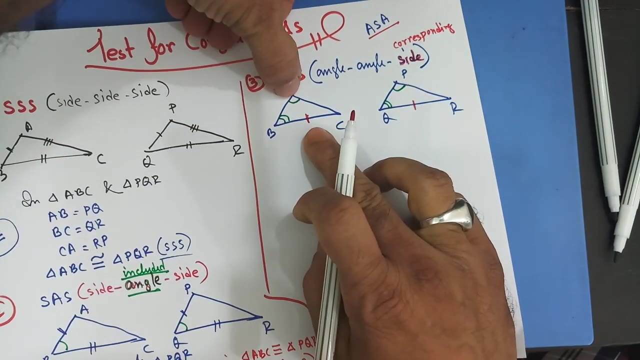 like that angle angle and this may mean that in between these two angle this side, in between these two angle this side, not necessarily okay. whenever it's a test of congruency, any corresponding side will do. i i may have this: see: one arc length drawn angles opposite side. is this one and one? 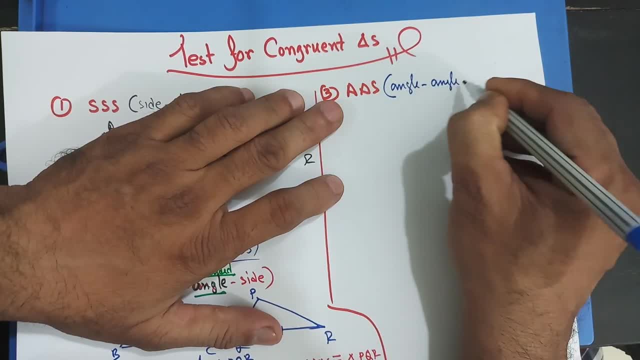 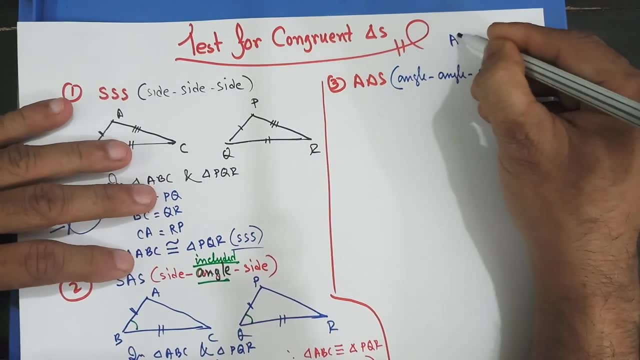 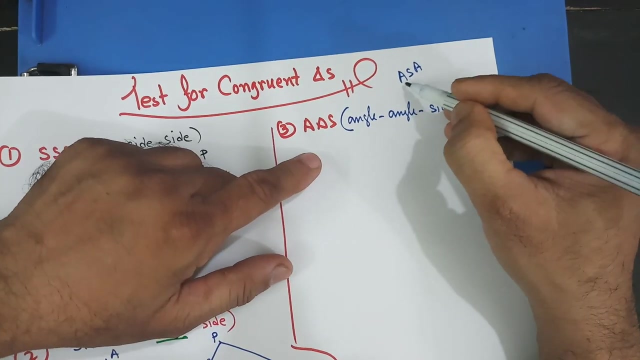 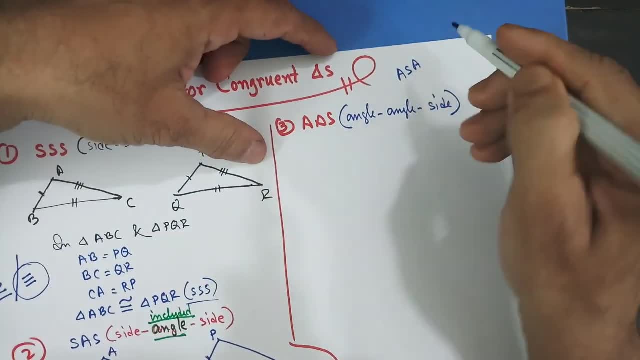 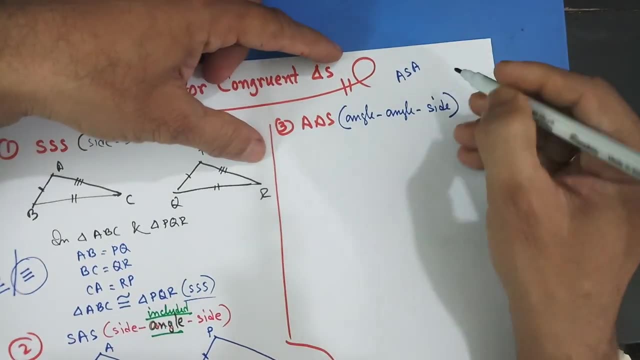 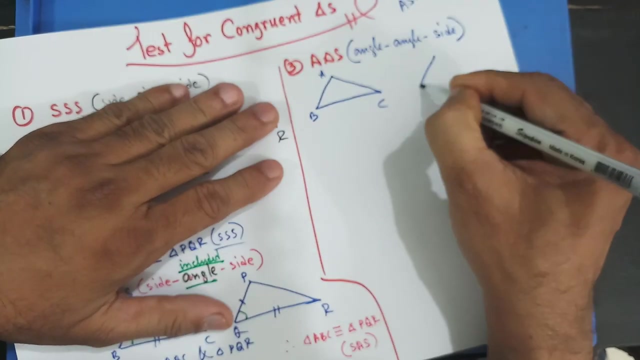 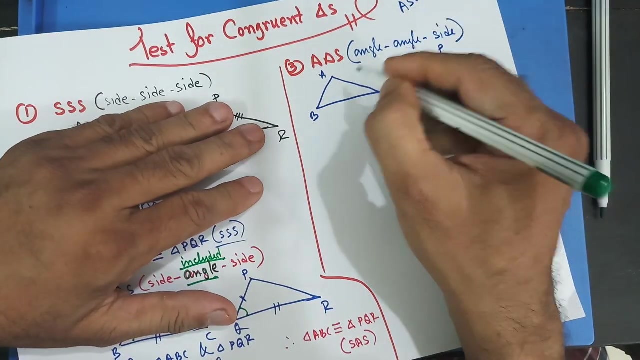 that side, corresponding side, but this is not the truth. okay, it should be corresponding side, but not included angle. if it's another side, it should be okay for congruency test. okay, let me give you this, this diagram first, then I'll explain. if I have ABC and over here I have PQR, okay, so over here, this angle a and this: 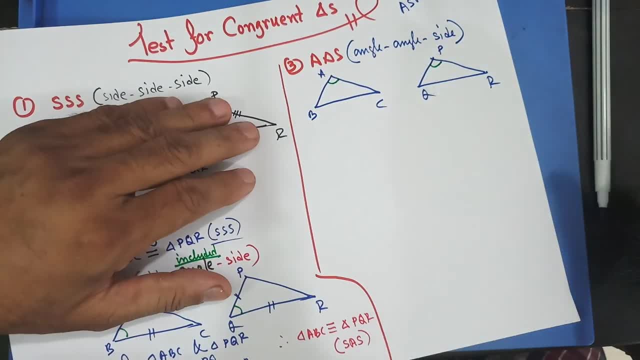 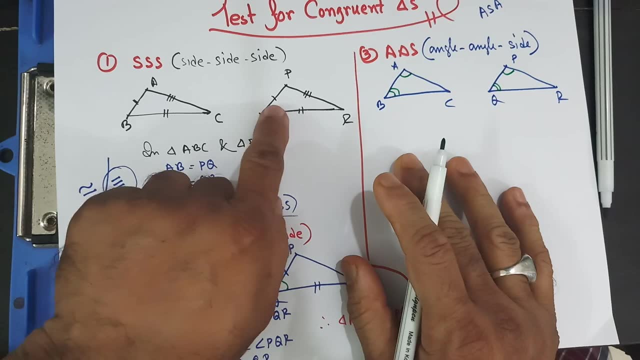 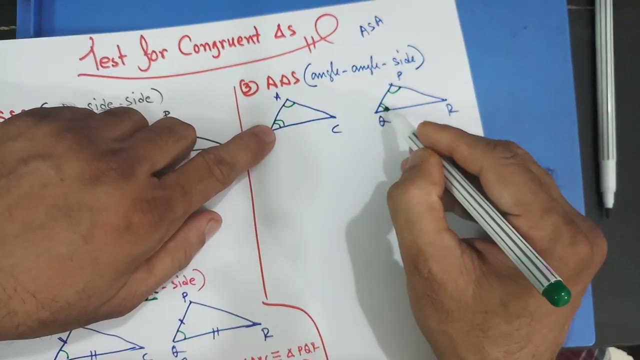 angle P, they are equal. and then I'm gonna use this B equal to Q, same as one bar, equal to one bar side over here for angle one arc length, one arc length, they are equal. and when i have two arc lengths, two arc lengths, these two are equal. so these two arc length. 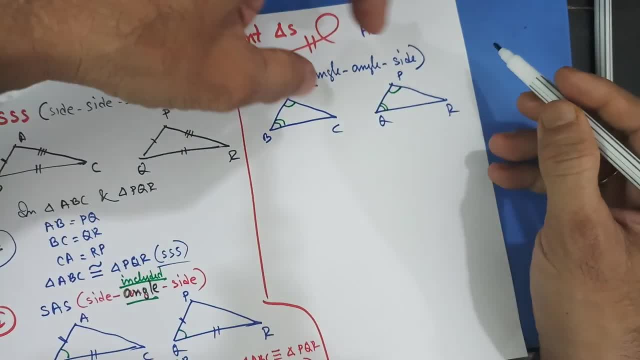 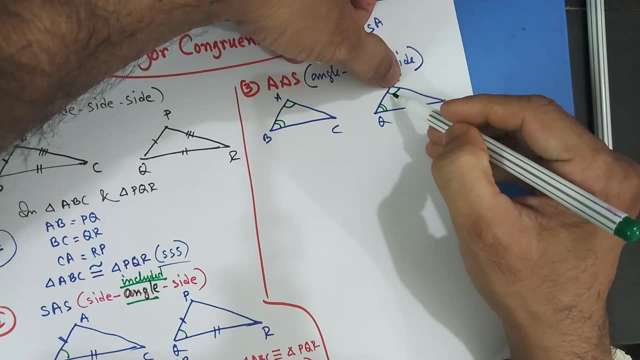 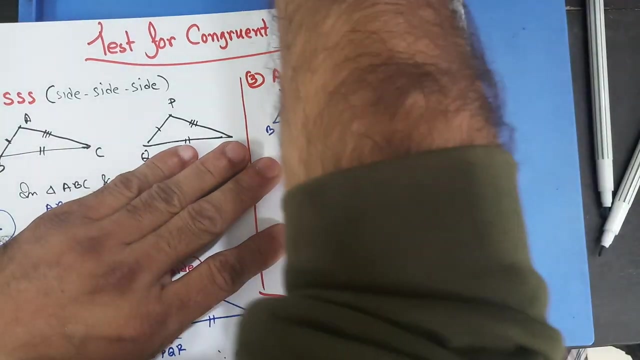 and one arc length angle are never equal in the same problem. same math um same diagram. if you have one arc length and another angle have one arc length. so these two are equal. and two arc lengths, two arcs length, they are equal. okay, now let's say i'm gonna say this side equal to this side, given 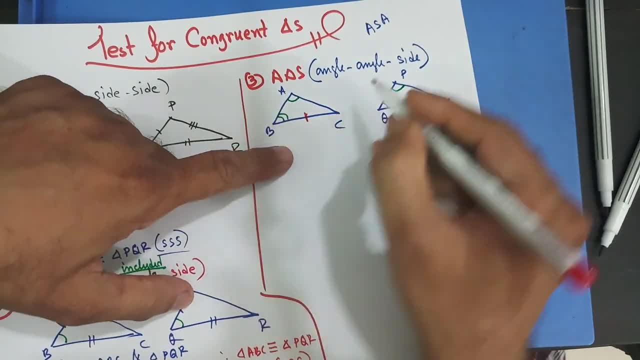 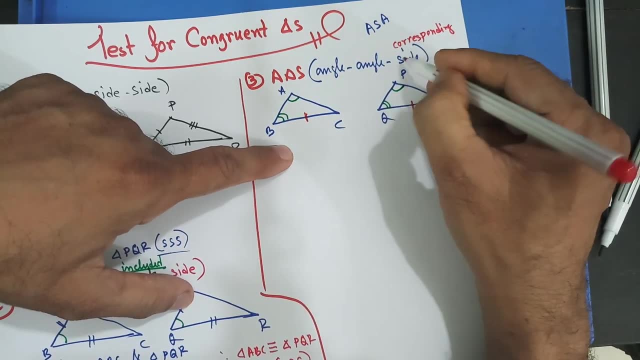 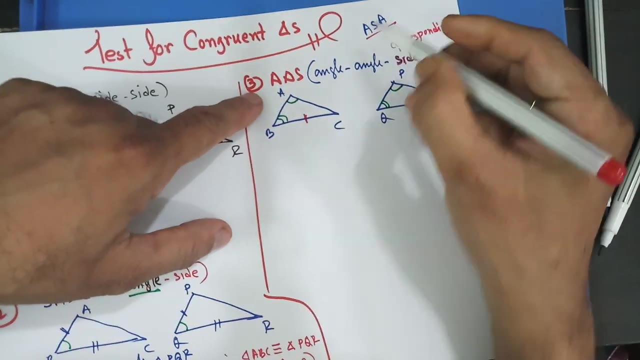 okay, it has to be corresponding side, angle, angle, corresponding side, not included angle. if it's included angle, it's gonna okay, okay, but corresponding side. so in this case, we're gonna say angle, angle and corresponding side. now if i put, like that, angle, angle and this may mean that, 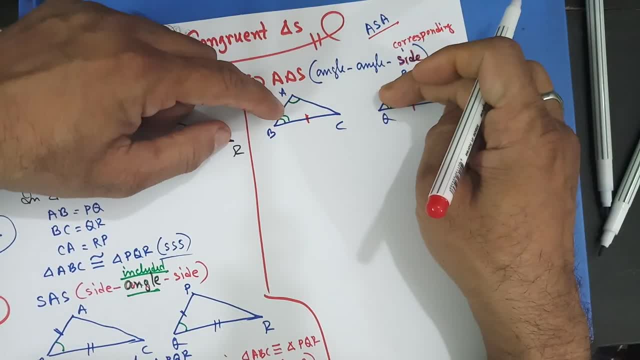 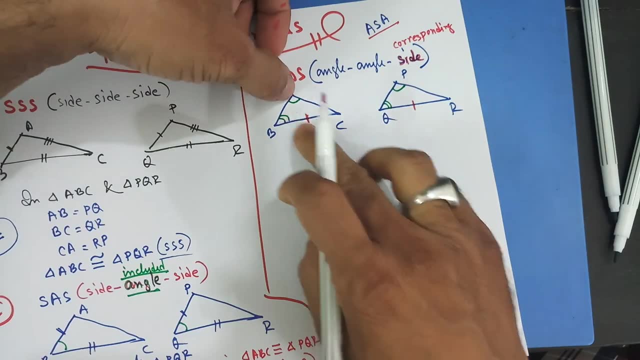 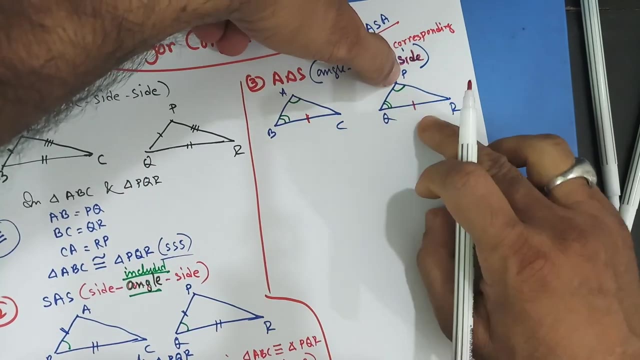 in between these two angle, this side, in between these two angle, this side, not necessarily okay whenever it's a test of congruency, any character. so i'm gonna say angle, angle and corresponding side will do i. i may have this see: one arc length drawn angles opposite side is this one, and one arc length angles opposite is this one. so these 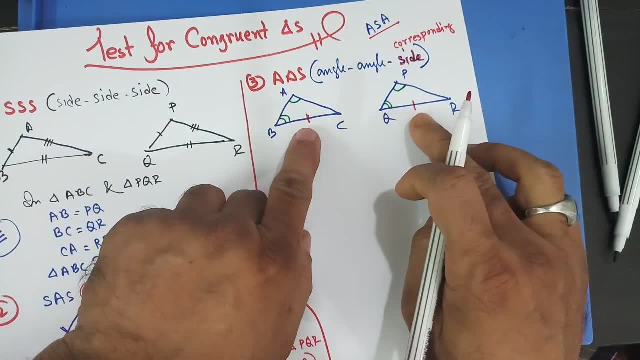 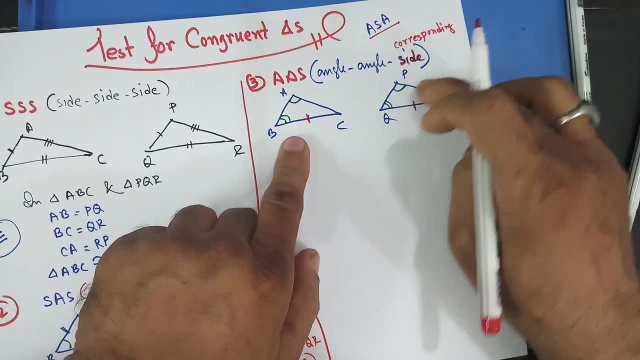 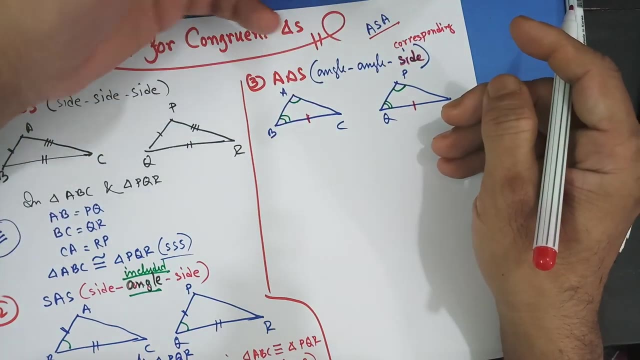 arc length angles. opposite is this one. so these are corresponding sides are equal. instead of that, if i had ca equal to rp, that should be okay too, because both of them are equal to the equal angles given. okay, or this included angles side should be okay too. so to just avoid the confusion, i write: 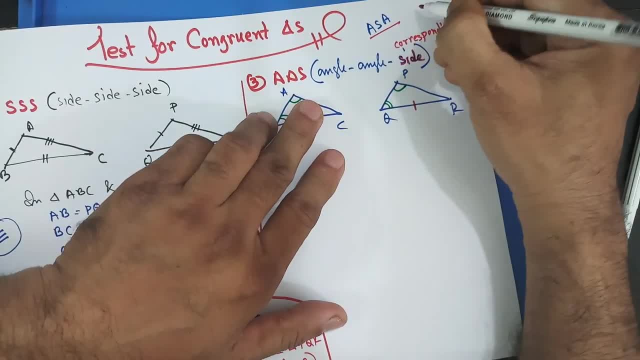 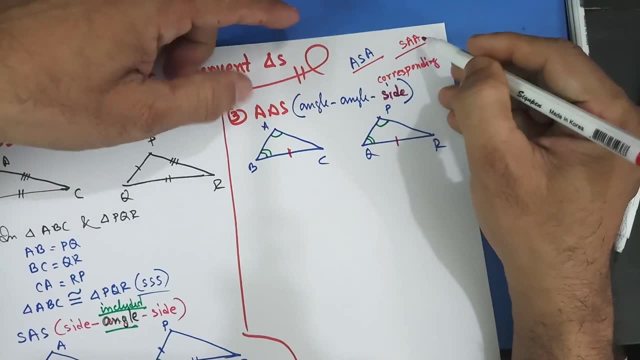 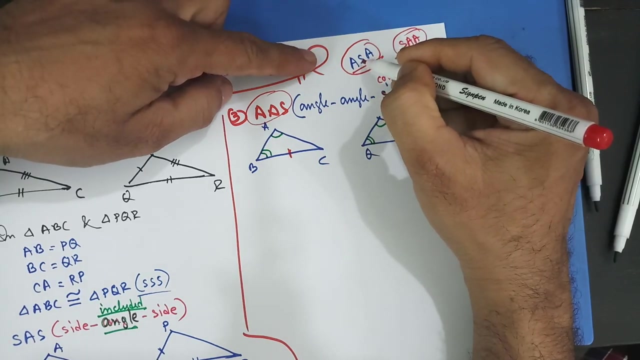 down: angle, angle 0. corresponding side. you may write down: saa, okay, it doesn't matter, okay, saa side, corresponding side. angle, angle: this or this should be okay, and to just avoid the confusion, we are not going to write like this: okay, i hope you understand that. so now, now what i'm going to do in triangle. 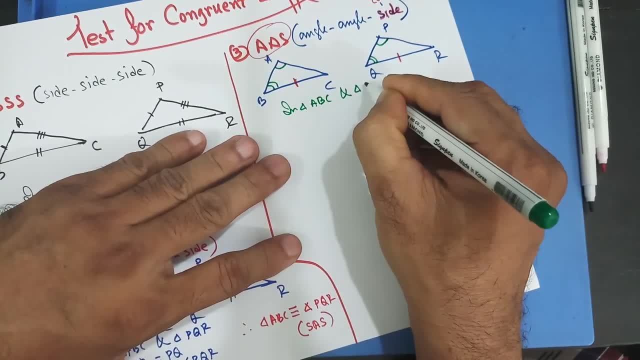 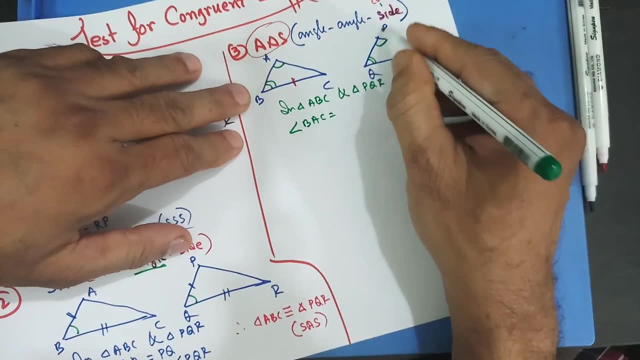 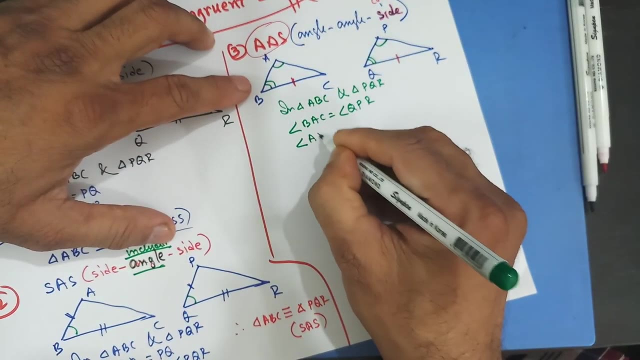 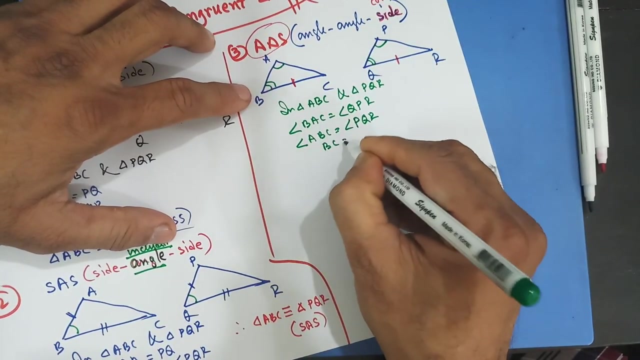 a, b c and triangle p q r angle b a c, b a c equal to angle q p r, q p r. this angles are given and then a b c, a b c equal to p q r, angle p q r and this side b c equal to q r given, so two: 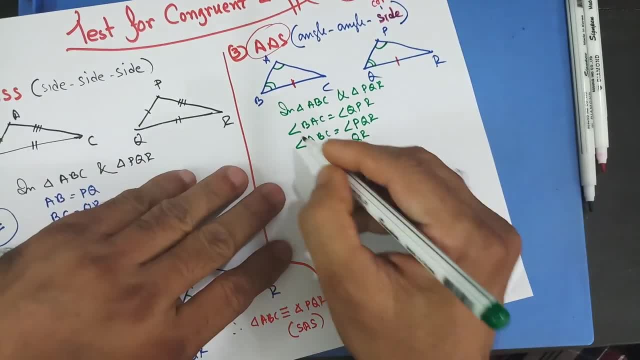 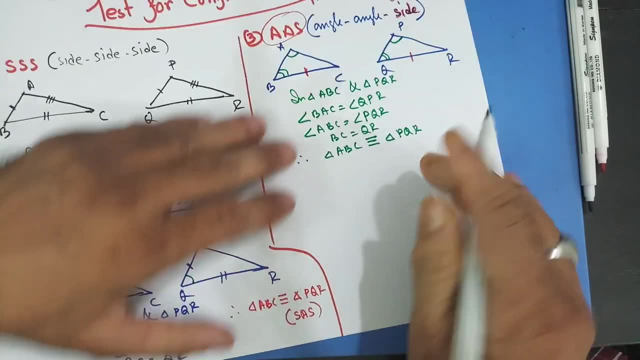 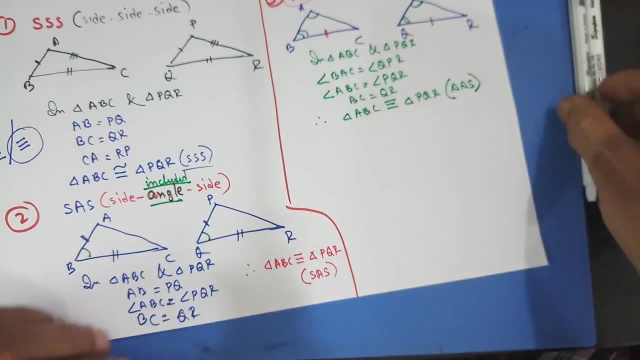 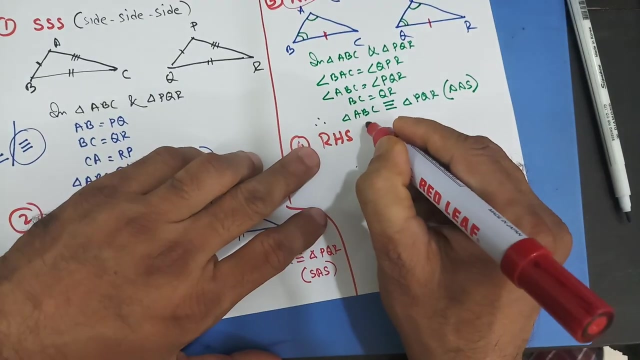 angles and one corresponding side is given, then we can write down: therefore, triangle a, b, c is congruent to triangle p, q, r, and, as before, we're going to write down: test of congruency: angle, angle, corresponding side. okay, that's the third one. now let's go for the fourth one. fourth one is r, h s. now r is. 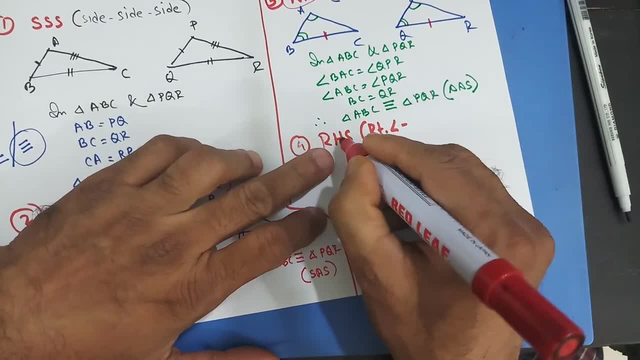 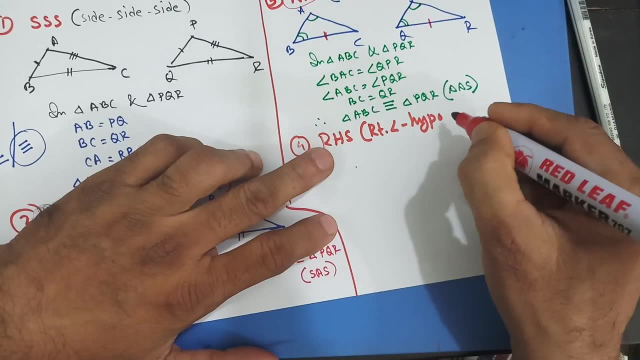 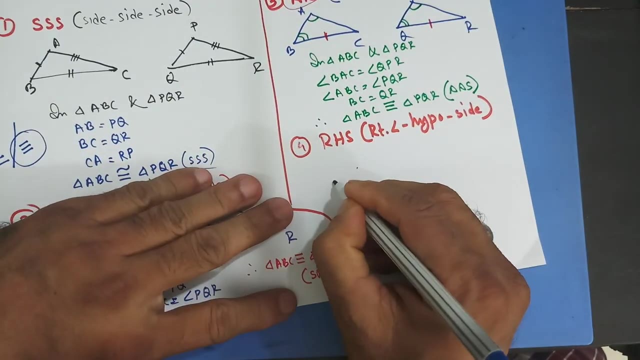 right angle, okay, right angle. and then h is hypotenuse, hypotenuse. hypotenuse means opposite of the right angle. triangle: uh, right angle and side is any corresponding side. okay, so when it's like that, let me, let me draw this right angle. so it must be a. 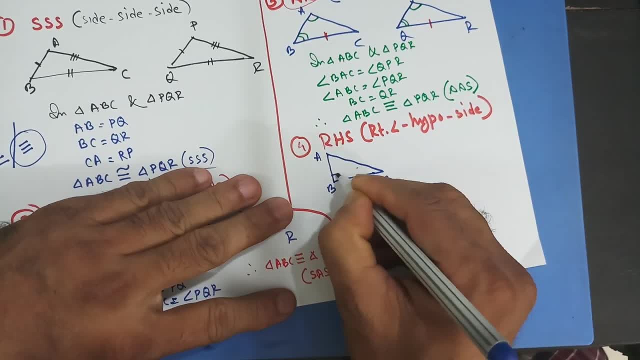 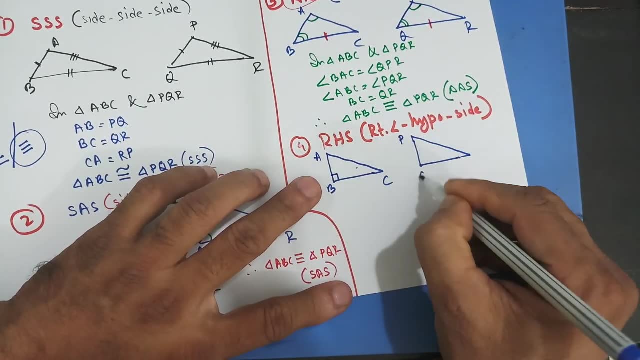 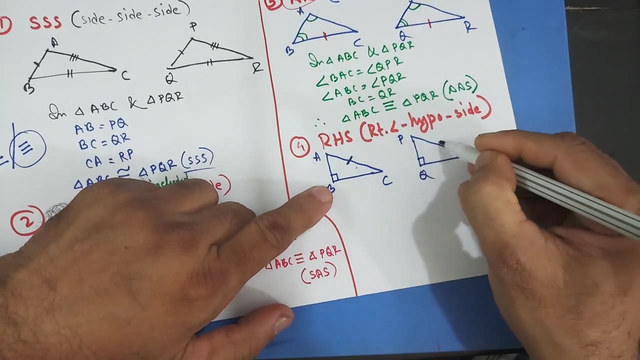 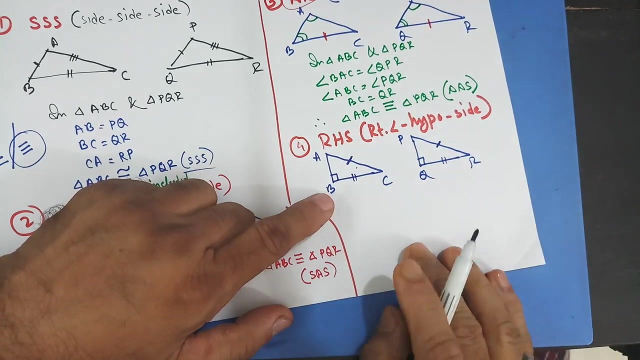 right angle triangle. so a, b, c. having this b a right angle. this is small square box represent right angle. then i have p, q, r and this is right angle. opposite of right angle is: this is hypotenuous, these hypotenuous are equal. and then take any other uh side. let me take this and this. okay, 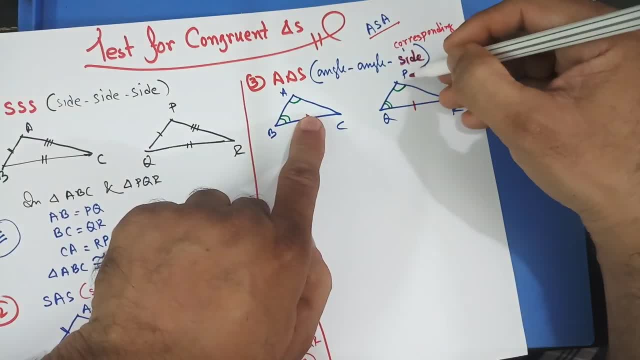 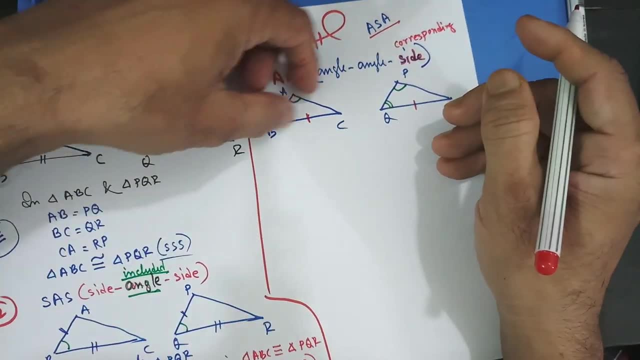 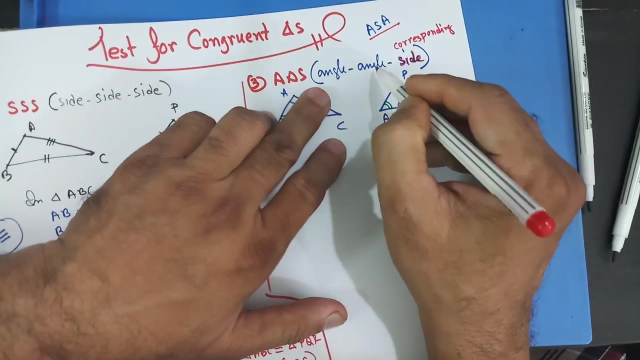 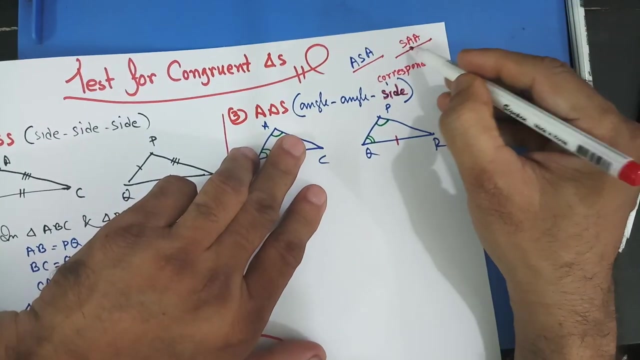 are corresponding sides are equal. instead of that, if i had c a equal to r p, that should be okay too, because both of them are equal to the equal angles given okay. or this included angles side should be okay too. so to just avoid the confusion- angle, angle, corresponding side- you may write down: s a a okay, it doesn't matter. okay, s a a side. 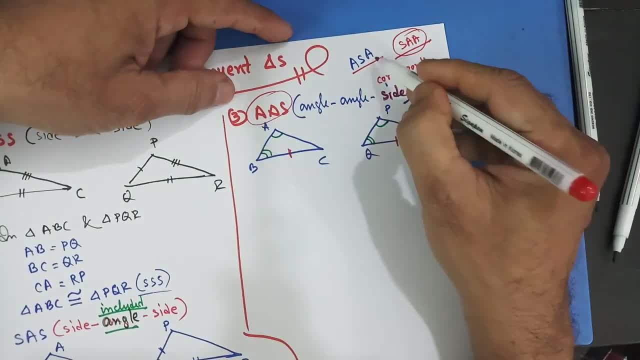 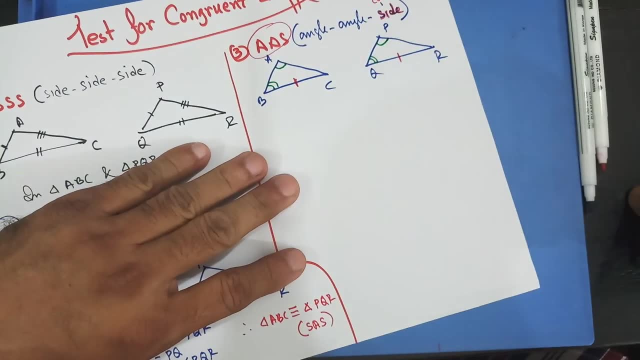 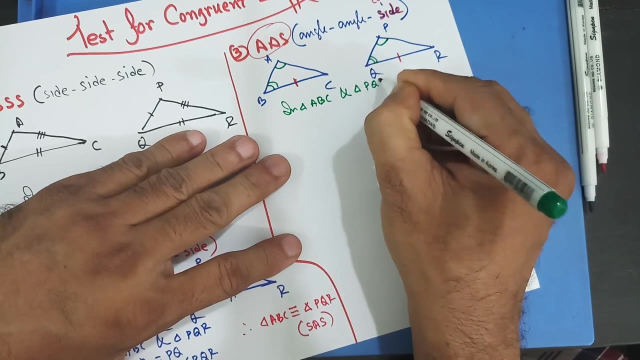 corresponding side angle, angle this or this should be okay and to just avoid the confusion, we are not going to write like this, okay, i hope you understand that. so now, now what i'm gonna do in triangle a, b c and triangle p, q, r. angle b a c. 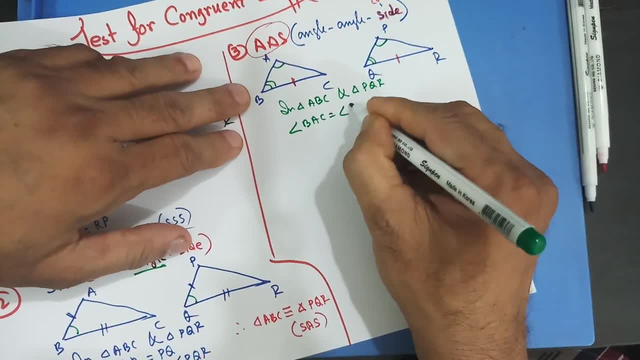 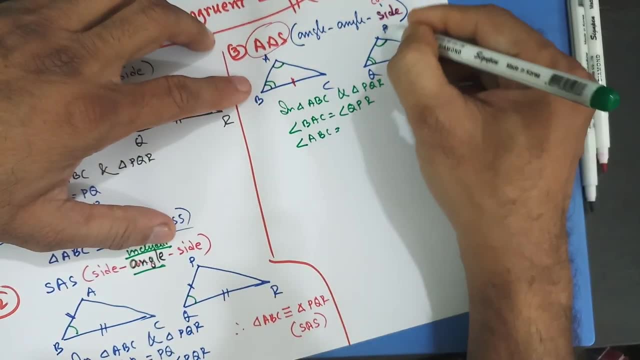 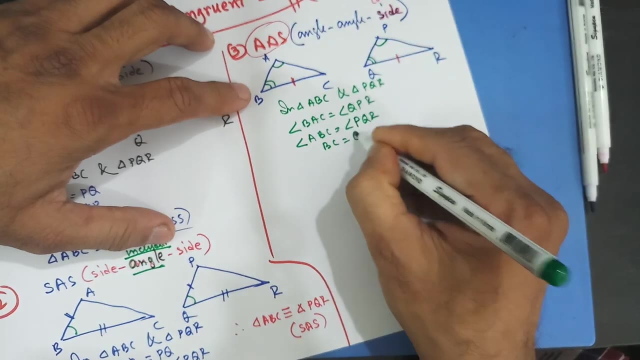 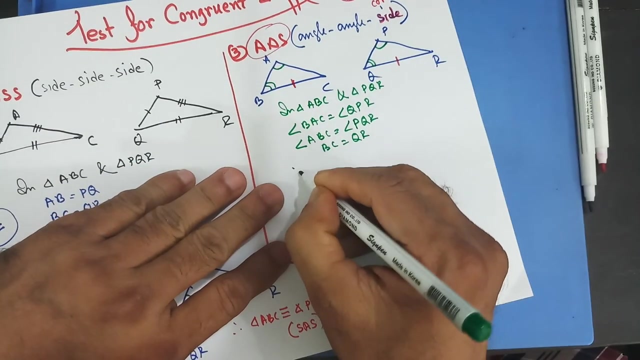 b, a c equal to angle q, p r, q, p r. this angles are given and then a, b, c, a, b c, equal to p, q r, angle p q r and this side, b c, equal to q, are given, so two angles and one corresponding side is given. then we can write down: therefore, triangle a, b c is congruent to triangle p q. 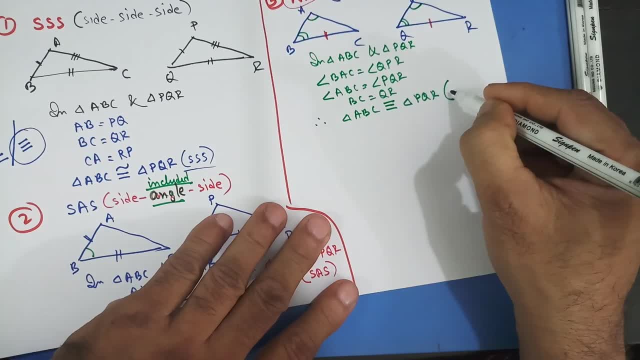 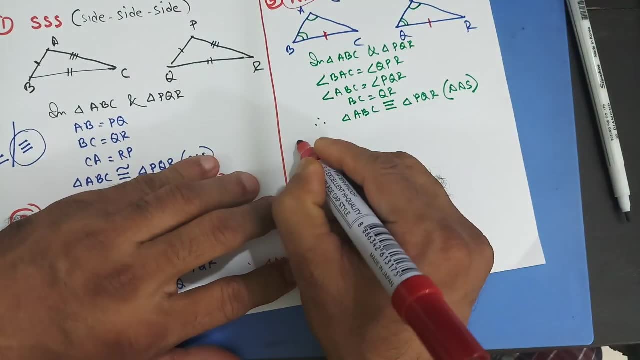 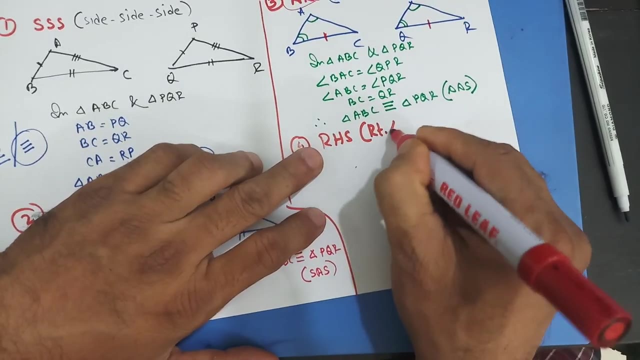 r and, as before, we're gonna write down test of congruency: angle, angle, corresponding side. okay, that's the third one. now let's go for the fourth one. fourth one is r, h s. now r is right angle, okay, right angle. and then h is hypotenuse. hypotenuse means 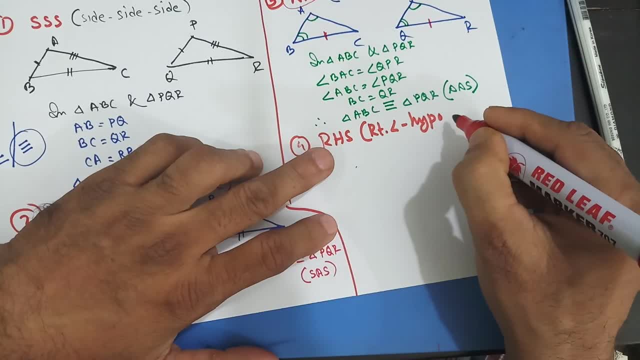 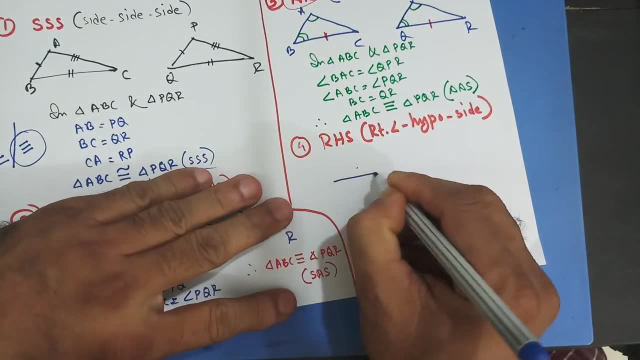 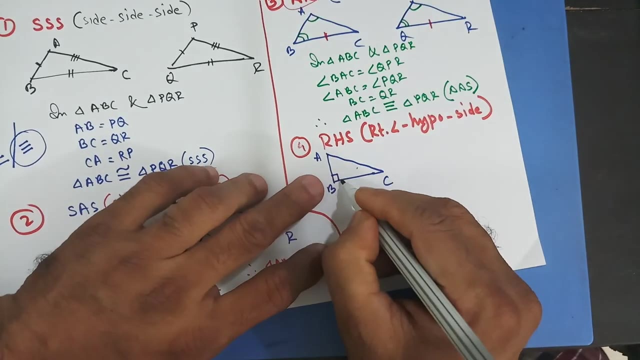 opposite of the right angle triangle. uh, right angle and side is any corresponding side. okay, so when it's like that, let me, let me draw this right angle. so it must be a right angle triangle. so a, b, c, having this b, a right angle. there's a small square box represent right angle. 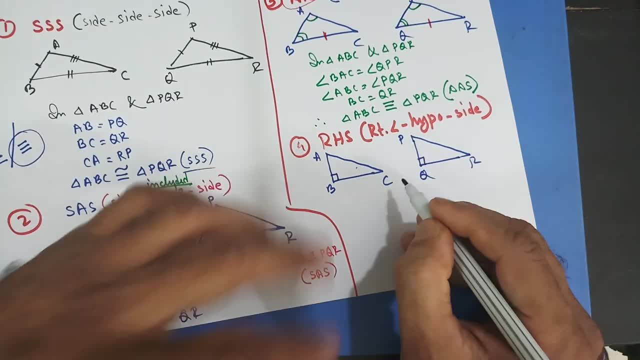 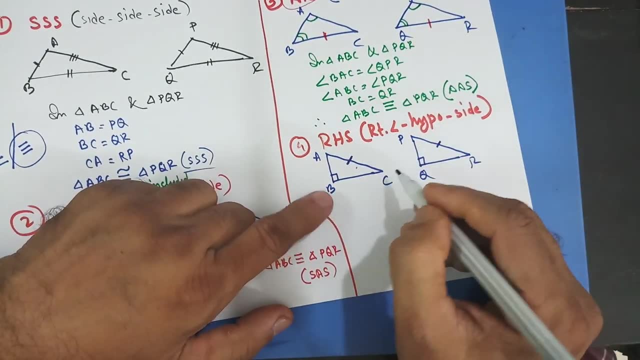 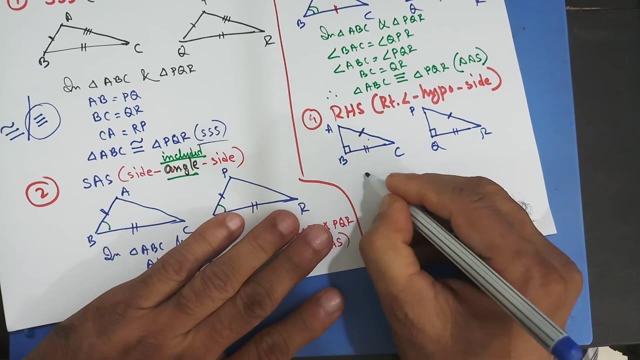 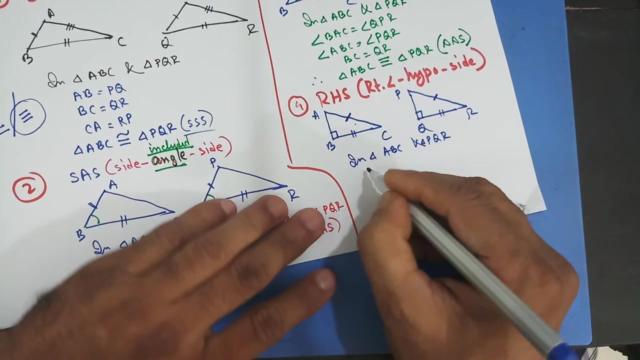 then i have p q r and this is right angle. opposite of right angle is this is hypotenuse. this hypotenuse are equal. and then take any other uh side. let me take this and this. okay, so this one in triangle a, b, c and triangle p q r. triangle p q r uh. angle b equal to angle q. 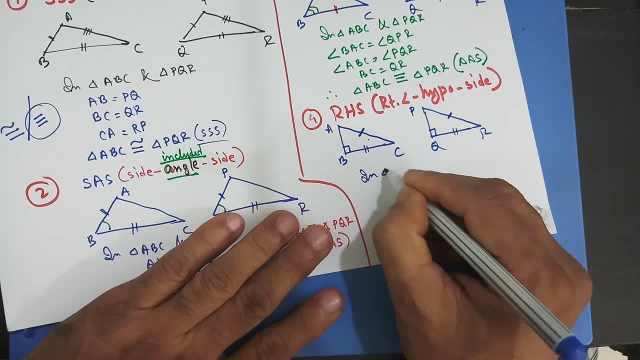 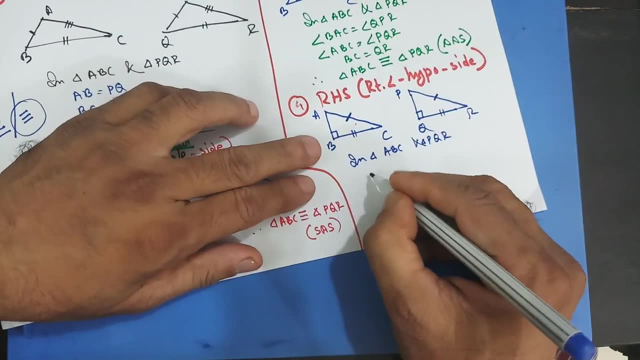 so b angle of triangle and triangle of triangle up m pq r triangle, pq r angle be equal to angle, q equal to 90 degree, that's for right angle, or for r- okay, right angle. and then hypotenuse is ac equal to 90 degree, that's right angle. or for r- okay, right, 감r. and then hypotenuos is ac equal to max. and then cef calm up and away, right. 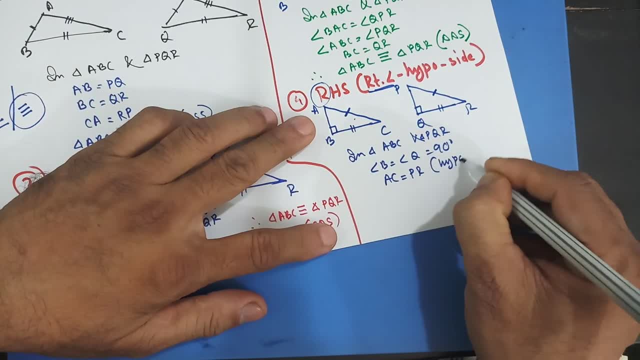 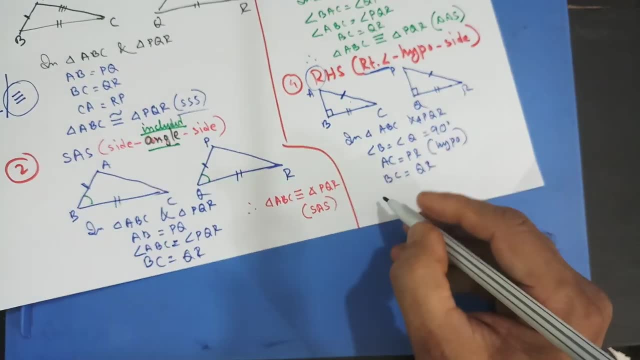 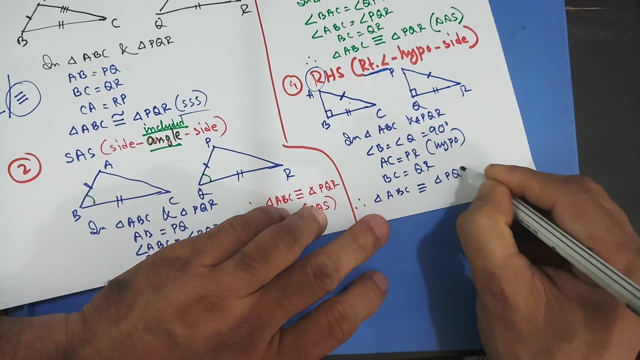 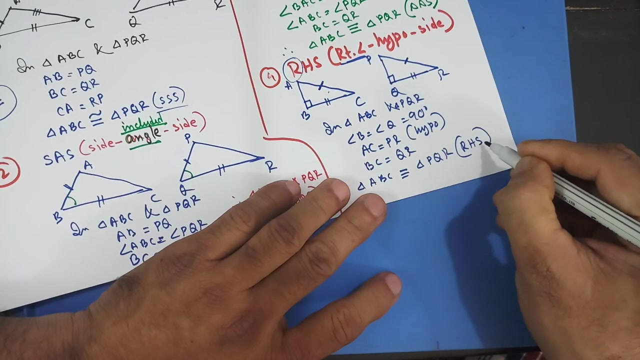 PR, okay, hypo or hypotenuse, and then corresponding side, BC equal to QR. and when I have that, I can write down triangle ABC. therefore, triangle ABC is congruent to triangle PQR and as usual, we're gonna write down: test of congruency is RHS, right angle, hypotenuse and corresponding side. now, when we have 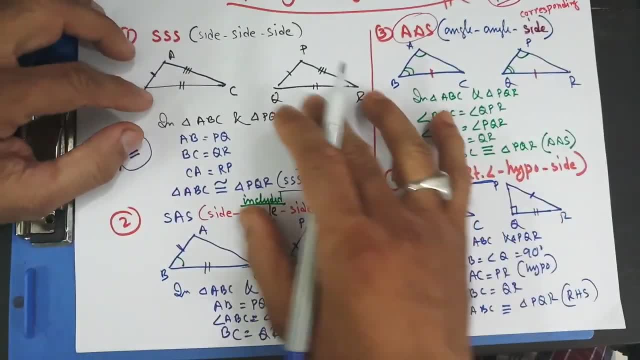 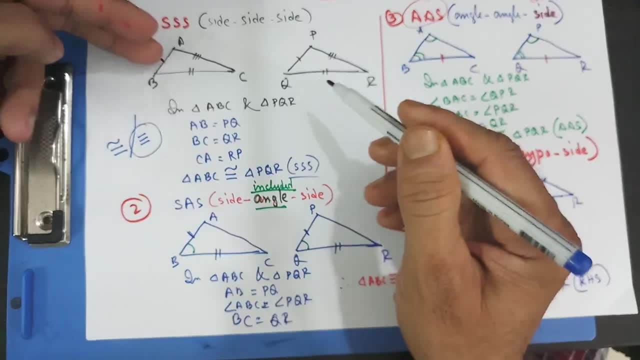 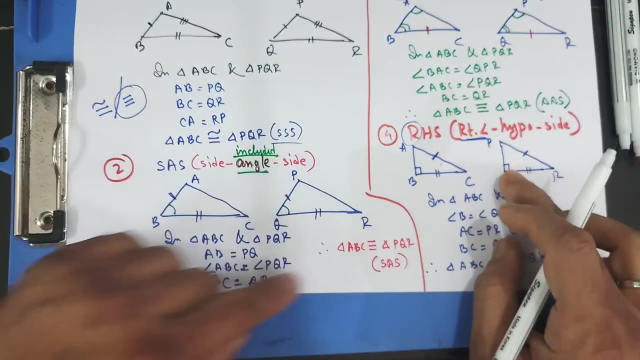 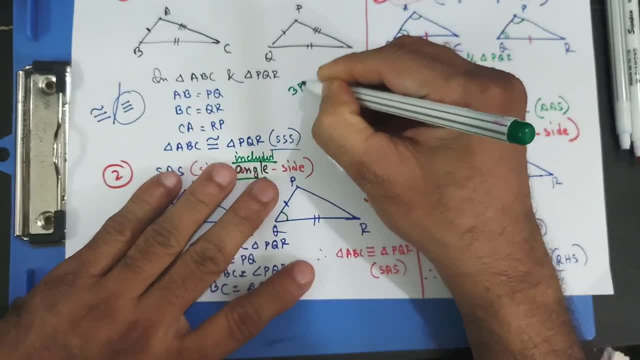 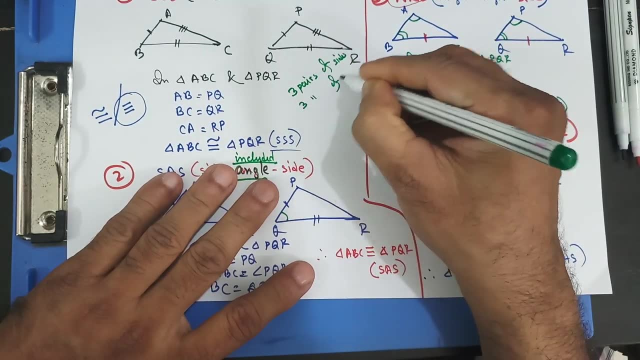 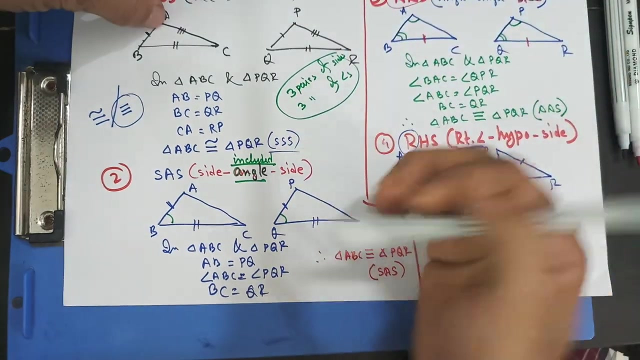 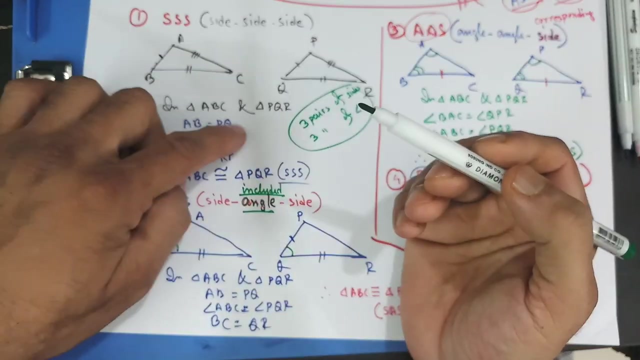 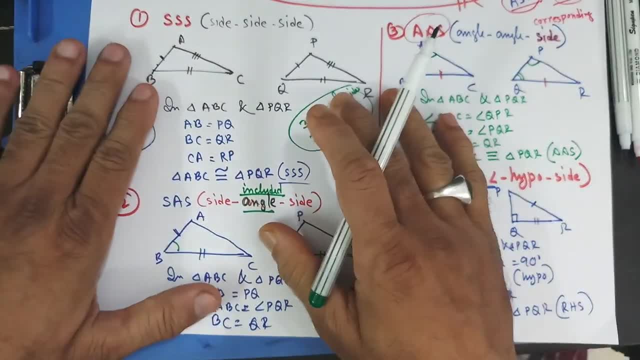 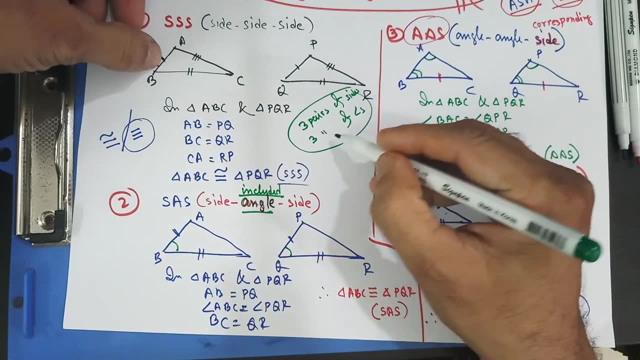 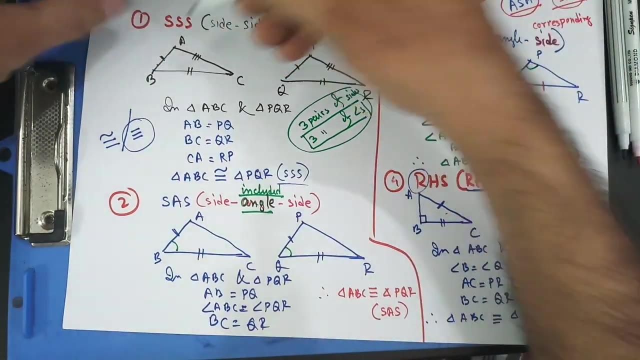 are equal. okay, when we have that, when you can prove that these triangles are congruent, these two triangles are congruent, having three equal sides, then we can say that therefore there are three angles, corresponding angles must be equal. so that means what I mean: that this angle A is opposite of the two bar. 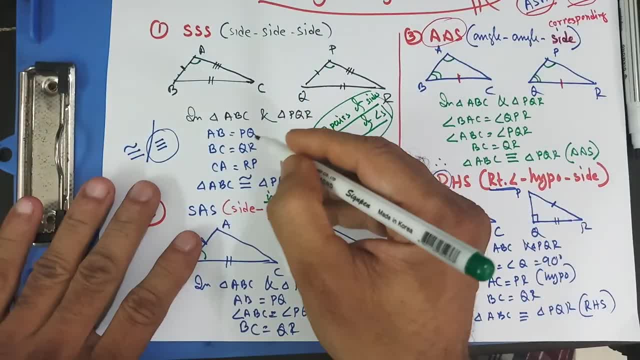 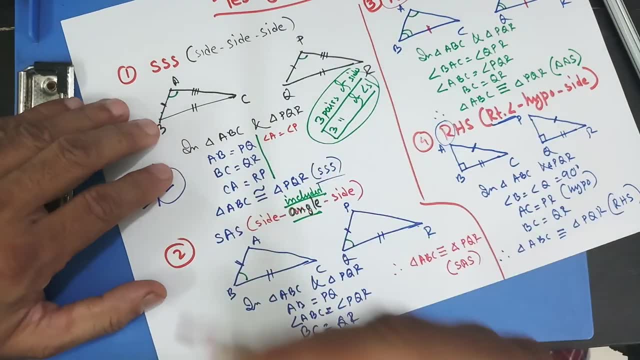 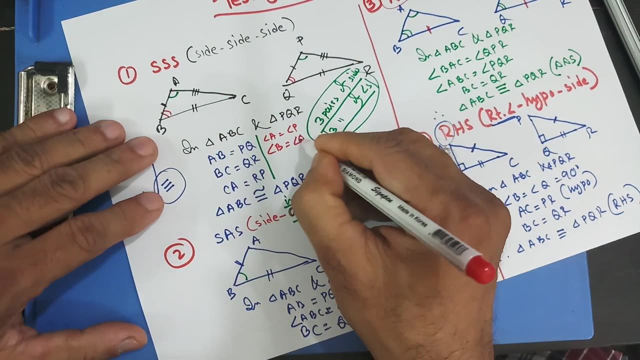 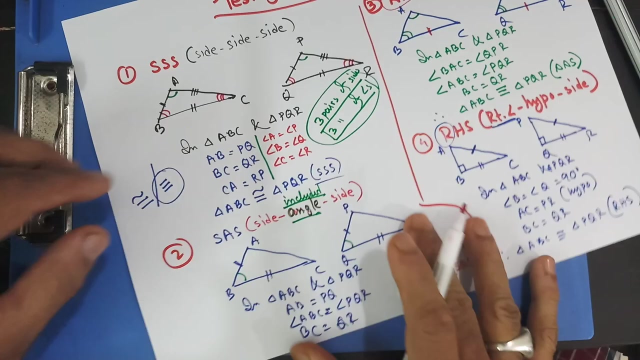 side opposite of two bar side, is this equal to that? so in this case, I can write down that angle A equal to angle P- that what we can derive- and angle B equal to angle Q, and, and angle Q and angle C equal to angle R, angle C equal to angle R. okay, so that's what we can. 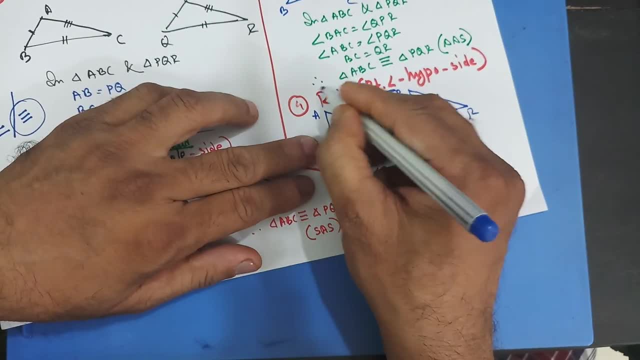 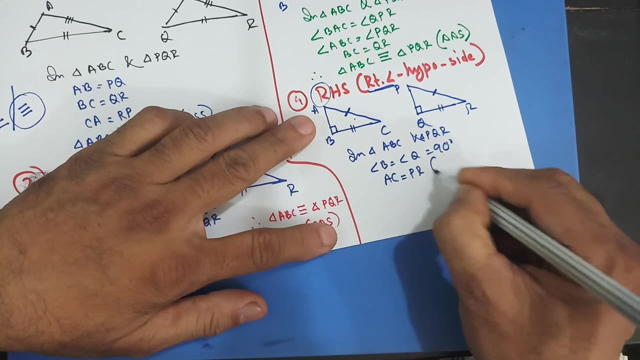 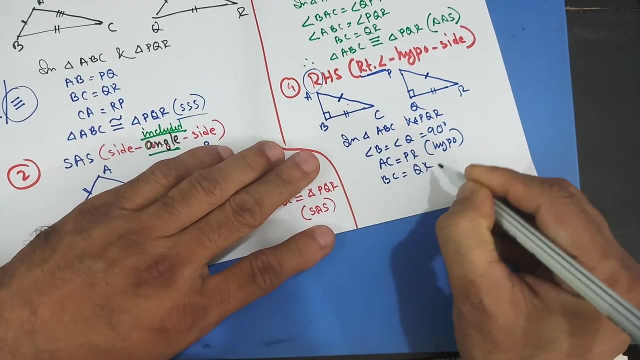 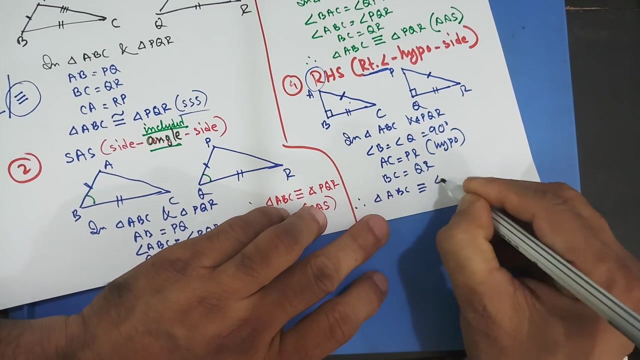 equal to 90 degree. that's for right angle or for r, okay, right angle. and then hypotenuse is a, c equal to p, r, okay, hypo, or hypotenuse. and then corresponding side, b, c equal to r. and when i have that, i can write down triangle a b c. therefore, triangle a b c is congruent to 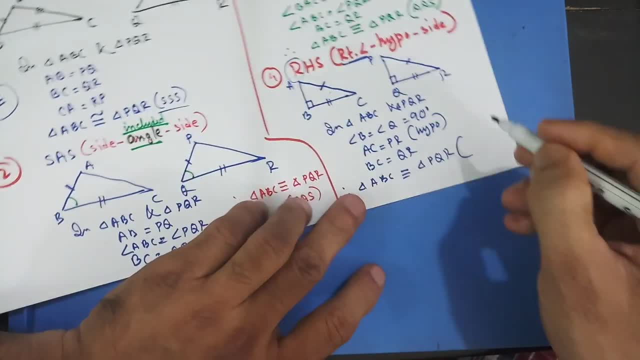 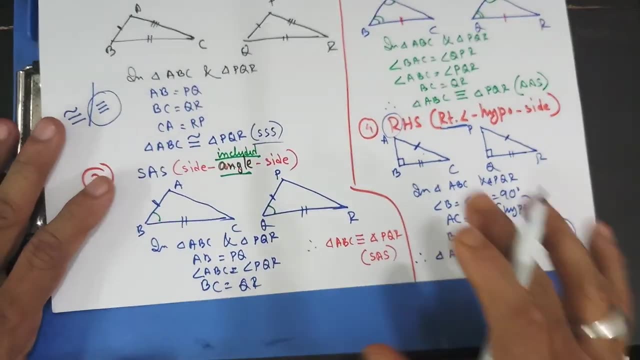 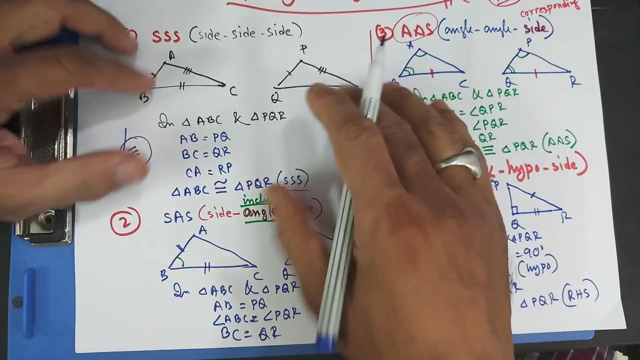 triangle p, q, r and as usual, we're going to write down test of congruency- is r, h, s, right angle, hypotenuse and corresponding side. now, when we have this test of congruency, okay, after proving that two triangles are equal, what can we achieve now? see that in these two triangles i have two. 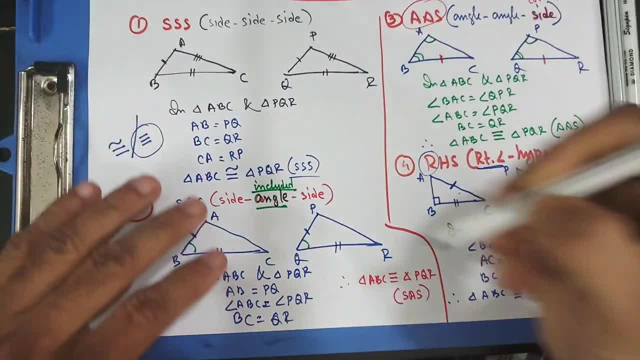 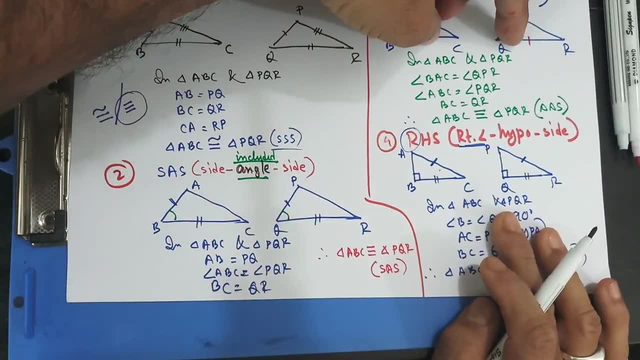 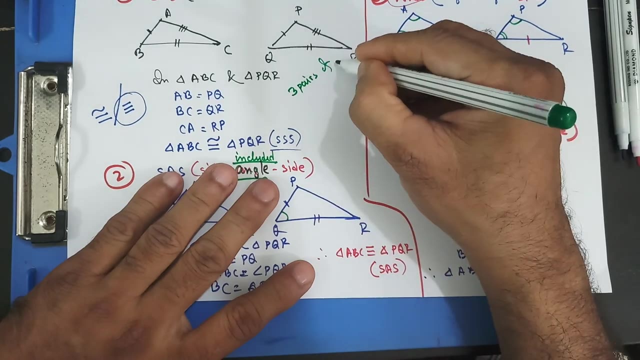 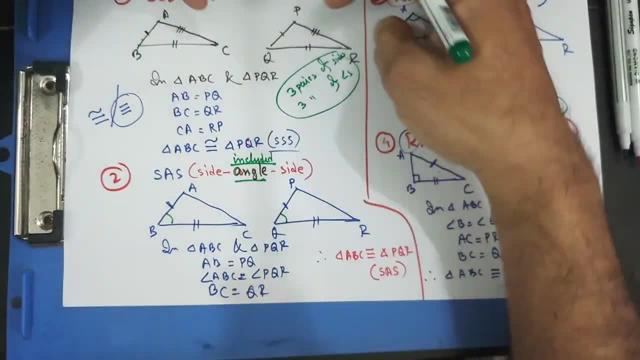 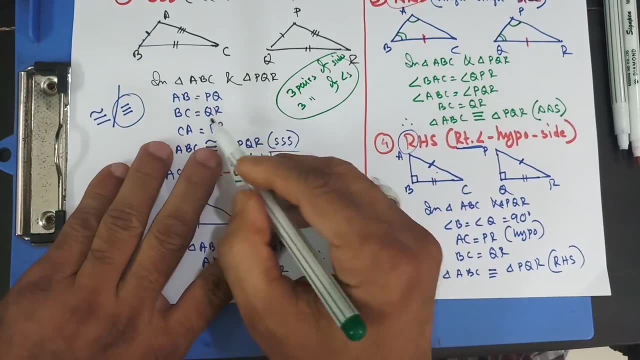 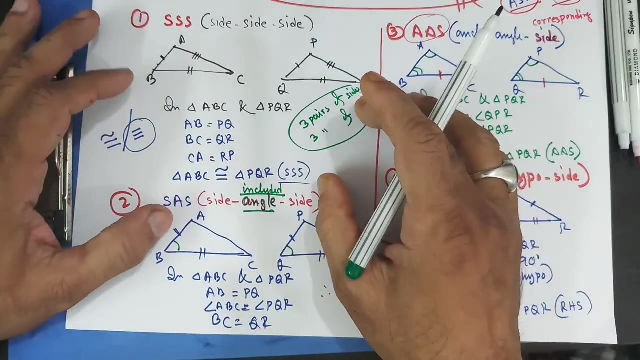 can you see that? one and one, that's one pair, two pair, three pairs of side and one pair of angle, pair of angle, three pairs of angles. okay, now, over here, we have proven that three corresponding pairs of sides are equal. okay, when we have that, when you can prove that these triangles are congruent. 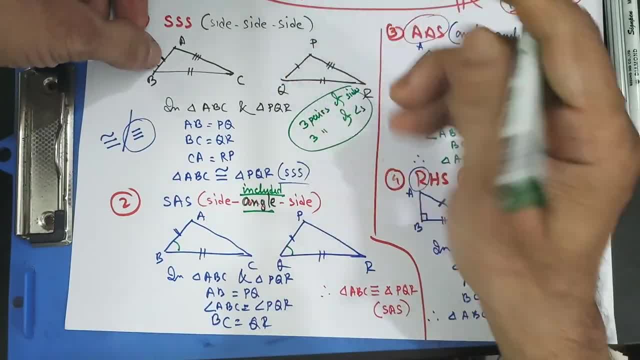 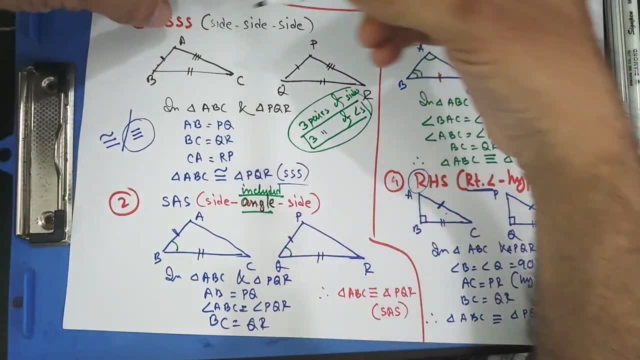 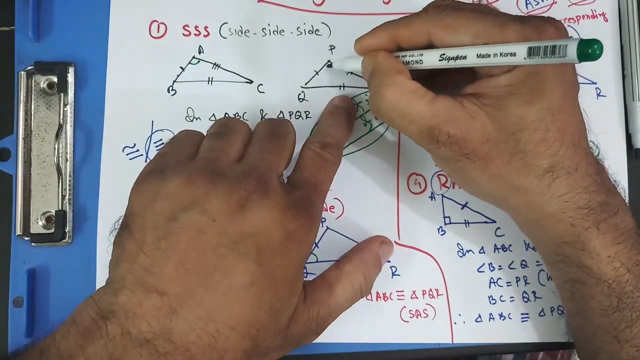 these two triangles are congruent, having three equal sides, then automatically i can say that therefore there are three angles, corresponding angles must be equal. so that means what i mean: that this angle a is opposite of the two bar side, opposite of two bar side. is this equal to that? 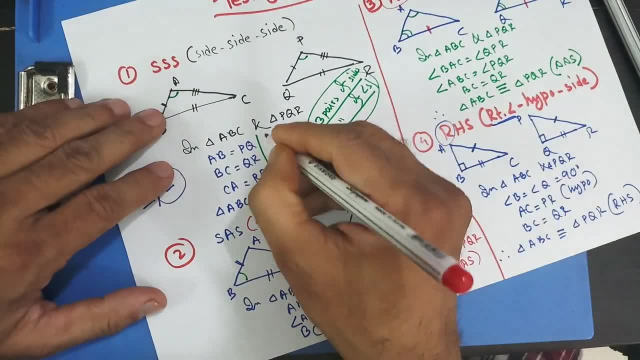 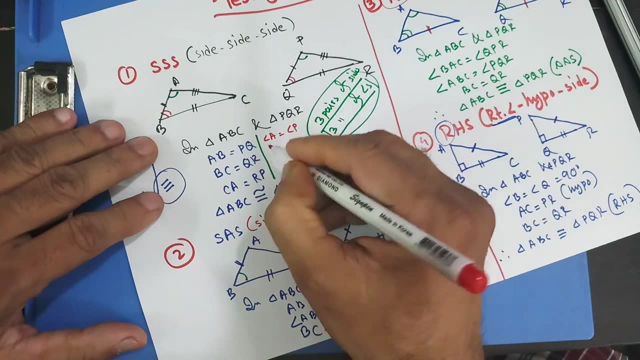 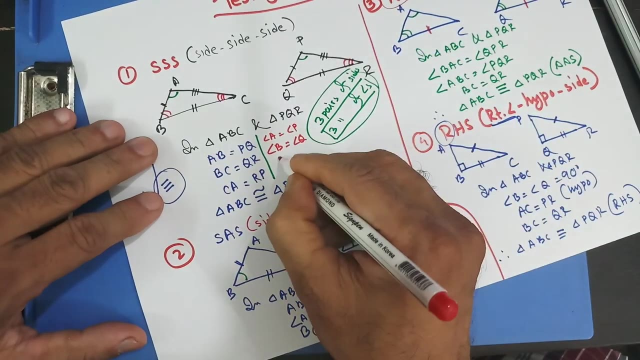 so in this case, i can write down that angle a equal to angle p, that what we can derive. and angle b equal to angle q, and and angle q and angle c equal to angle r, angle c equal to angle r. okay, so that's what we can achieve. 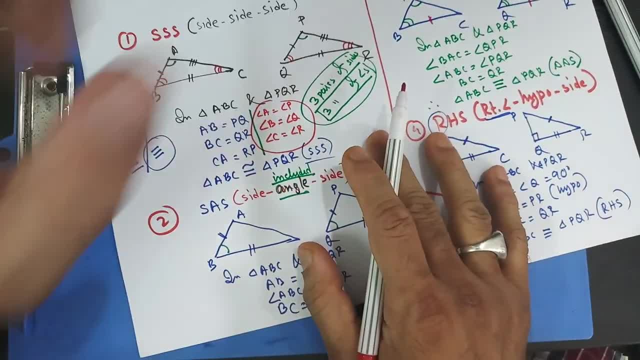 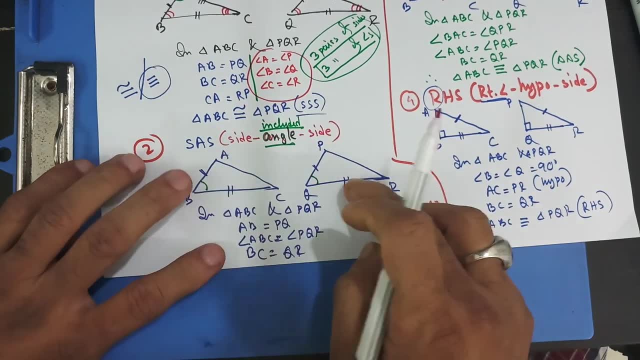 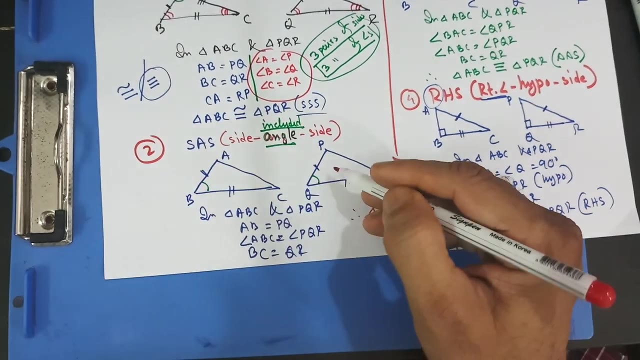 achieve as soon as we prove that these two triangles are congruent. now, same thing over here. I have proven that two pairs of sides, uh, with the, with the, with the information given, two sides, uh, two pairs of sides, are equal to each other and one pair of angle equal to each other. so, since I already have taken or given two sides, 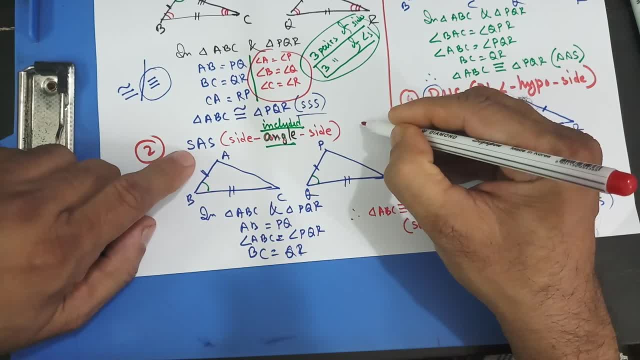 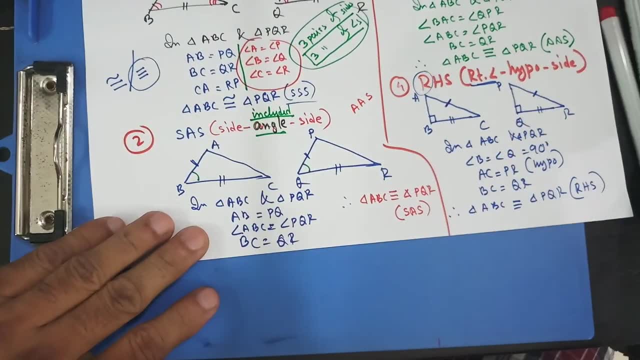 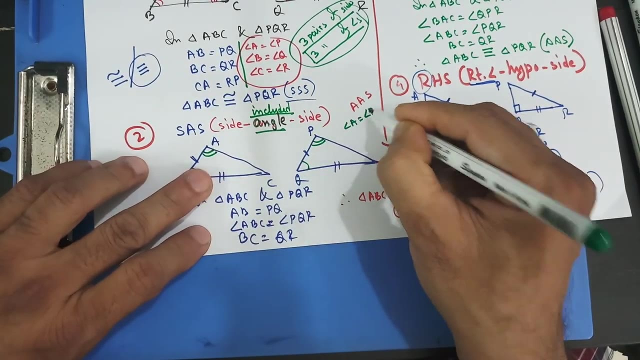 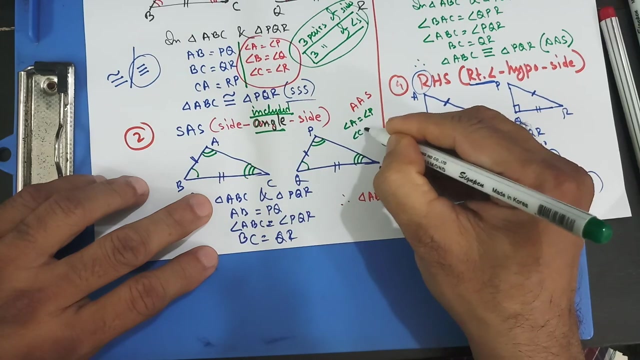 then one angle E is equal. then I can show that other two angles and one side are equal. that means I can go for this one, this angle equal to this angle. that means angle A equal to angle P- this one already was considered or given. then angle C equal to angle R, angle C equal to angle R and this side is left. so this: 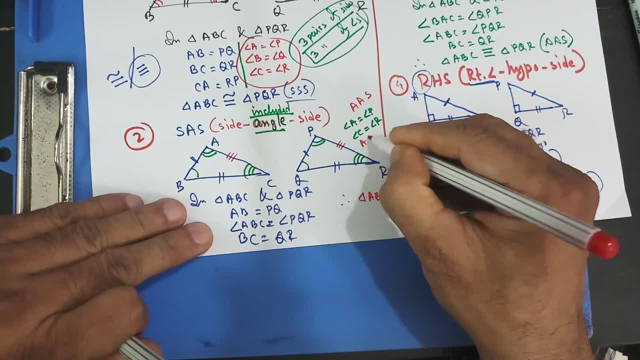 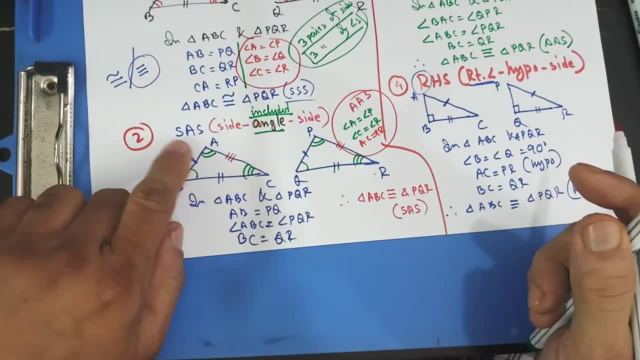 side equal to this side is left. now this side is left, this side. why? because now one side, that is, it's between one a and one side of the side. that's what we can say. so AC equal to P? R. okay, so we from this SAS our side. 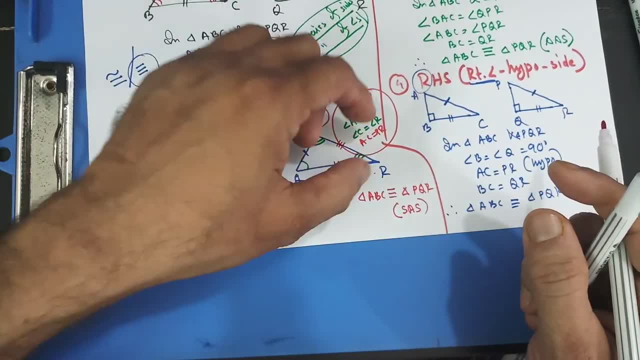 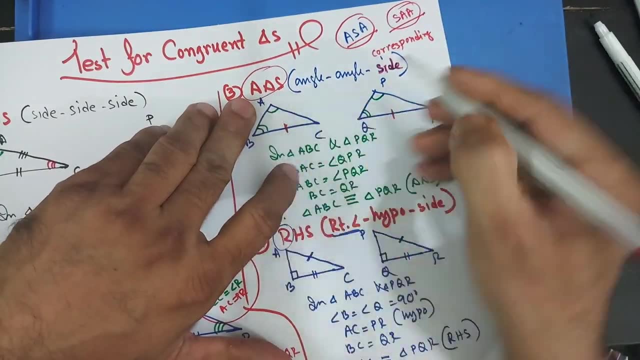 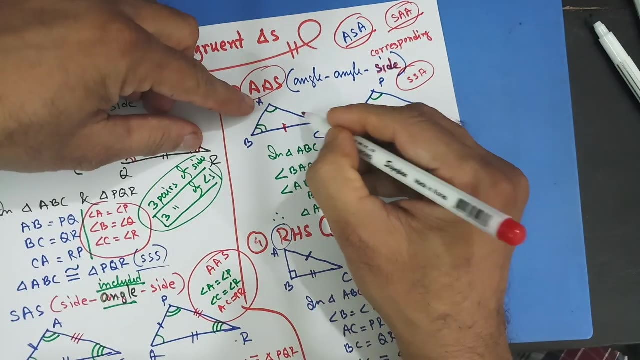 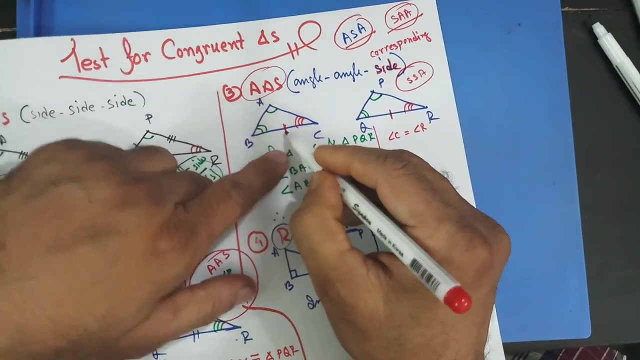 included angle side. we can derive this information that they are equal. now, when we are coming to this, we use two angles and one side, so we can prove other two sides and one angle are equal to each other. so I have taken this, so this left this angle and this angle left, so I can say angle C equal to angle R and then 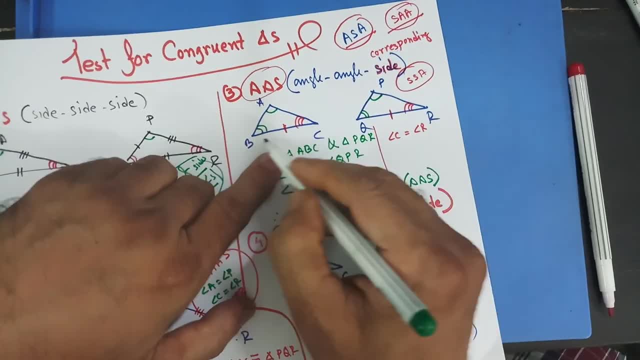 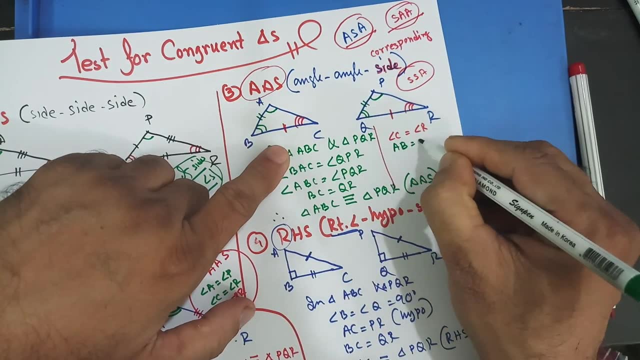 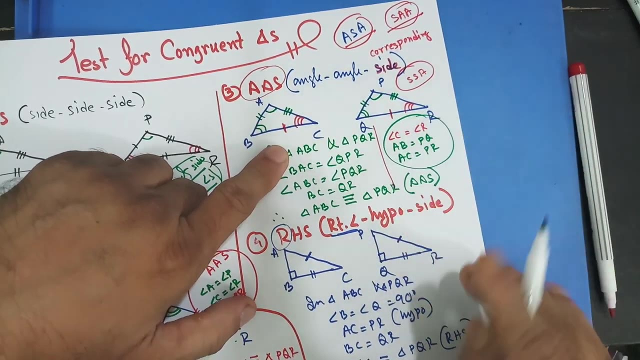 since this one was already taken, it was given BC equal to QR. so I can say: this AB equal to PR, PQ, a B equal to PQ and this AC equal to PR, AC equal to PR. okay, so that's them, and over here I have right angle, one angle, so I can just 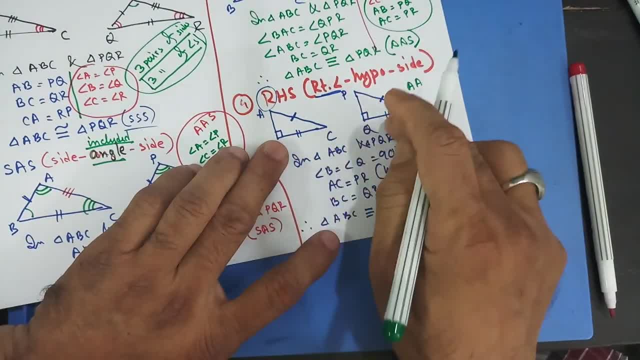 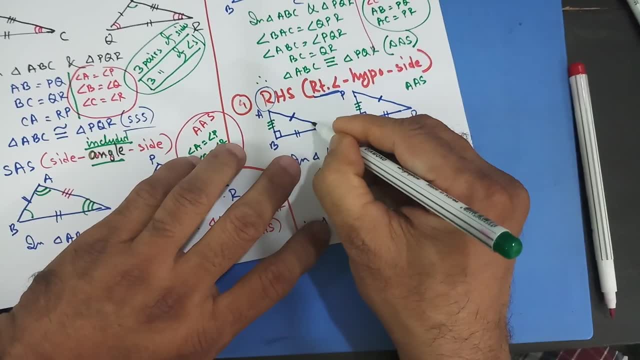 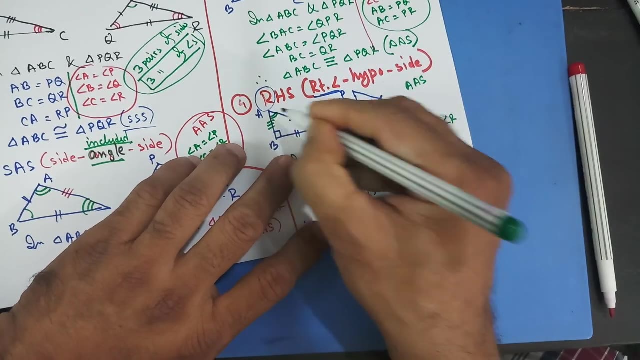 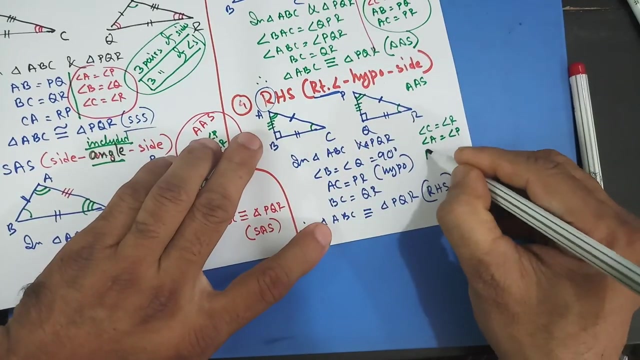 say that other two angles, corresponding angles, are equal to each other, and then two sides are given, so third side has to be equal. so i can say angle c equal to angle r, angle c equal to angle r from these two triangles and angle a equal to angle p, angle a equal to angle p and ab equal to. 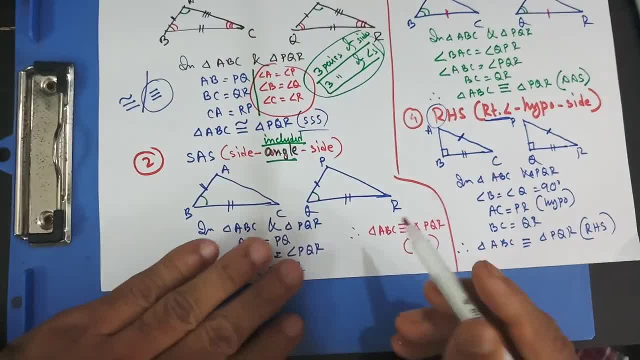 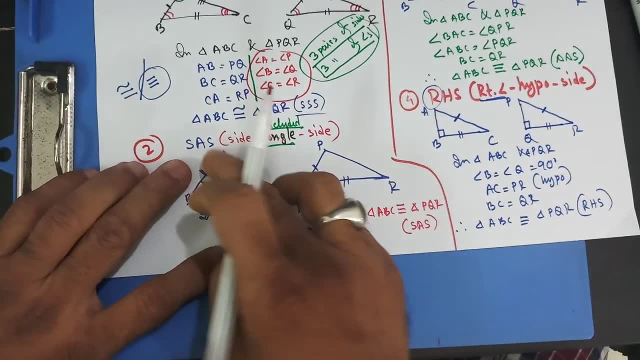 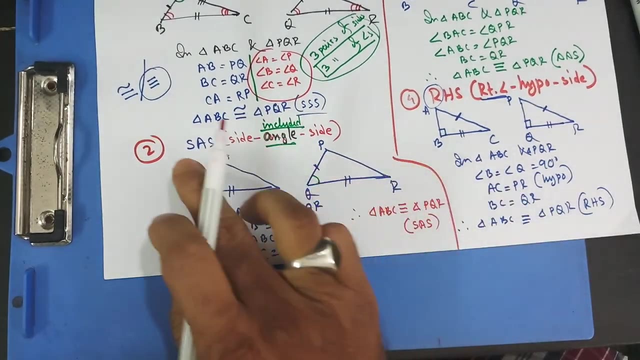 as soon as we prove that these two triangles are congruent. now, same thing over here. i have proven that two pairs of sides, uh, with the, with the, with the information given, two sides, uh, two pairs of sides, are equal to each other and one pair of angle equal to each other. so, since i already have 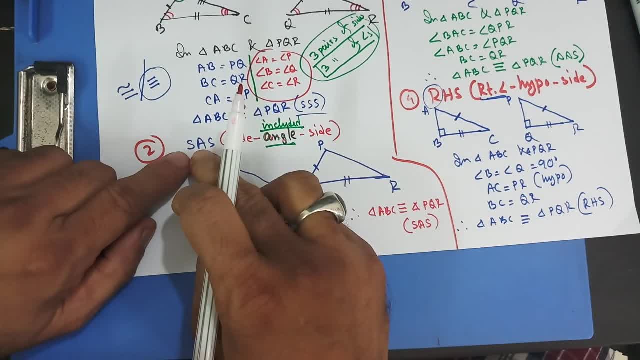 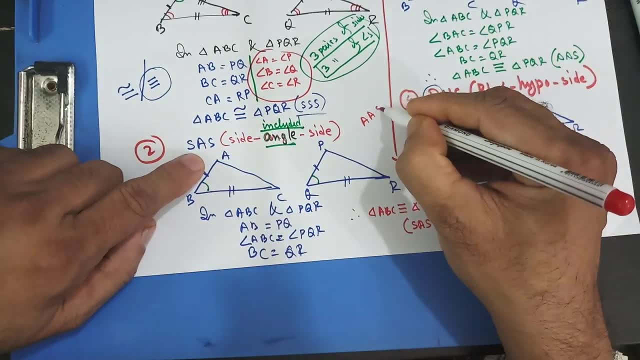 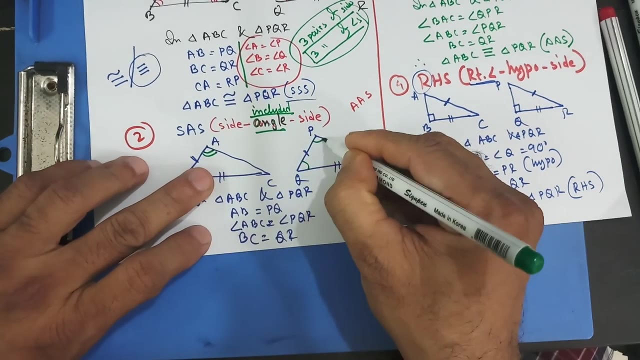 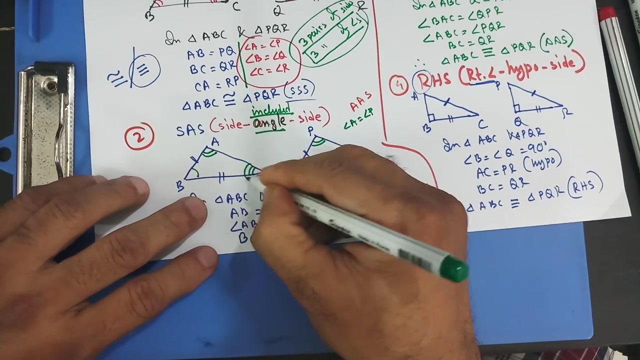 taken um or given, two sides are equal and one angle is equal, then i can show that other two angles and one side are equal. that means i can go for this one. uh, this angle equal to this angle. that means angle a equal to angle p. this one already was considered or given. then angle c equal to angle r. 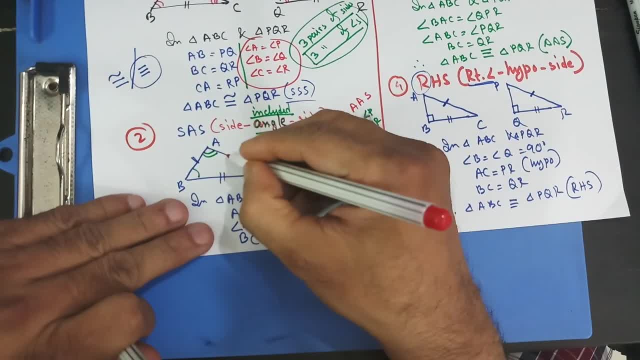 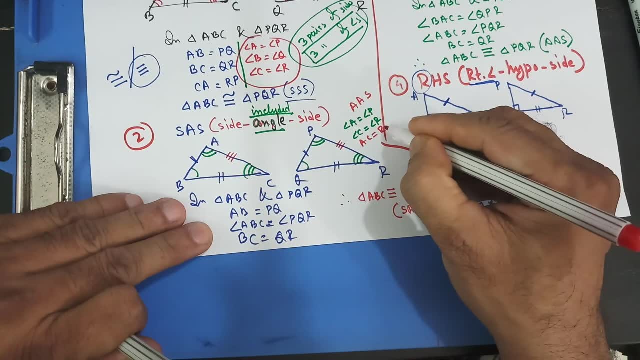 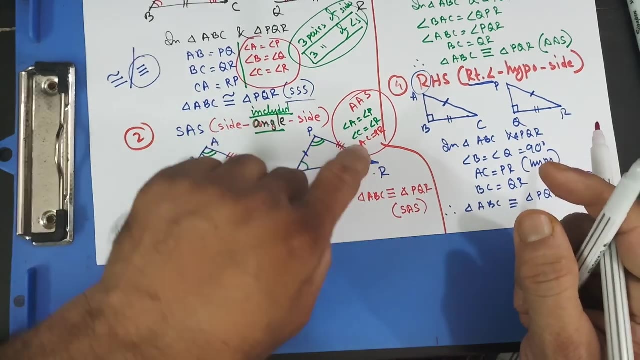 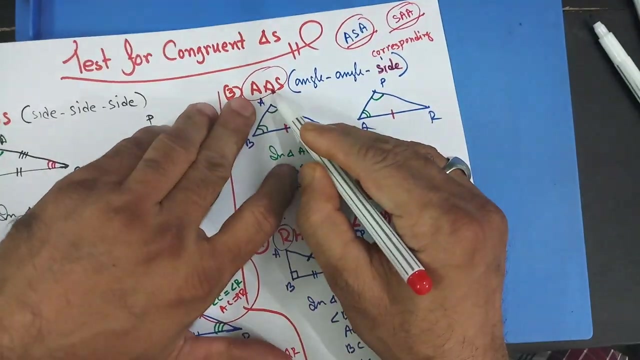 angle c equal to angle r and this side is left. so this side equal to this side. that's what we can say. so ac equal to pr. okay, so we, from this s a s our side included, angle side, we can derive this information that they are equal. now, when we are coming to this, we use two angles and one side, so 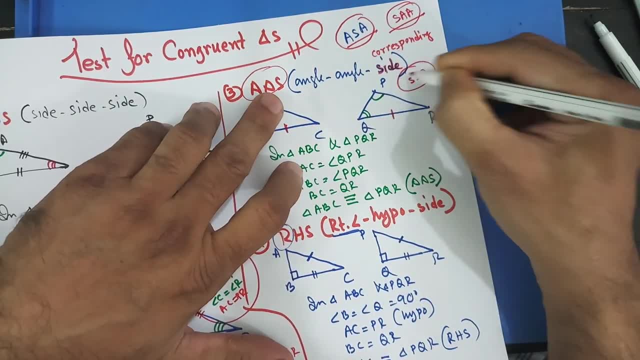 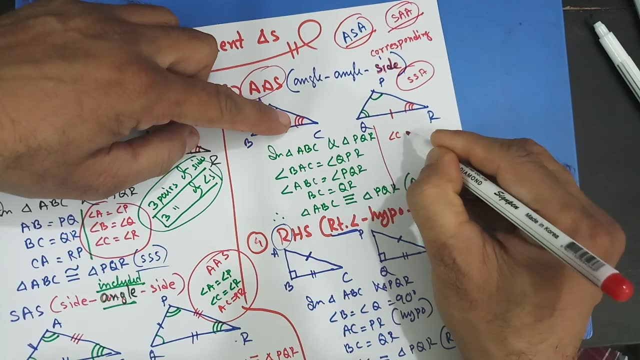 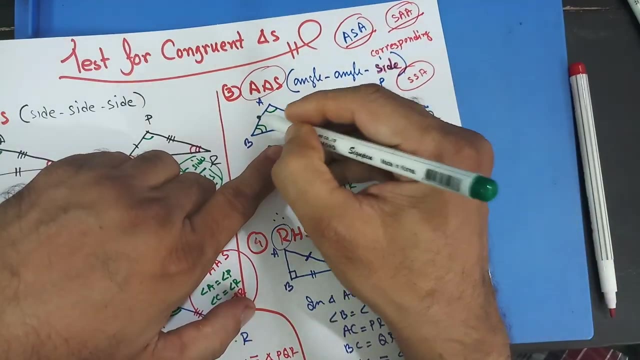 we can prove other two sides and one angle are equal to each other. so i have taken this, so this left, this angle and this angle left, so i can say angle c equal to angle r. and then, since this one was already taken, it was given bc equal to qr, so i can say this: a- b equal to p, r, pq, a- b equal to. 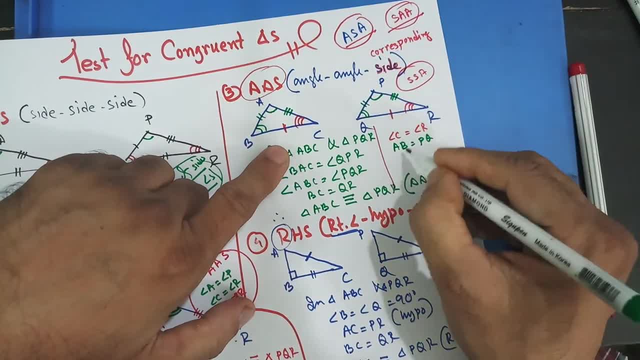 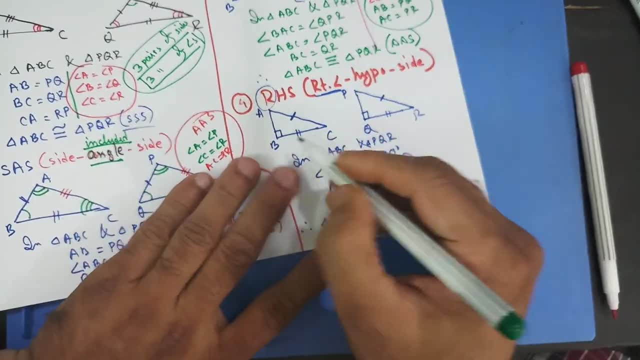 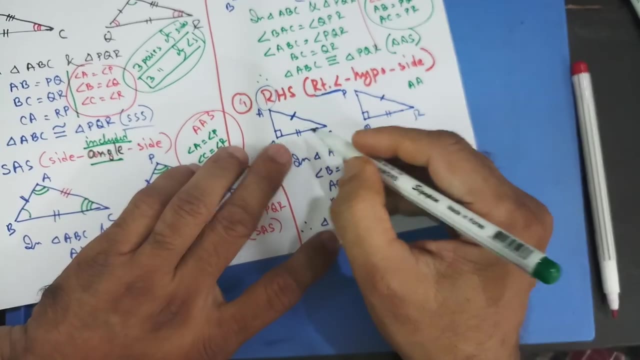 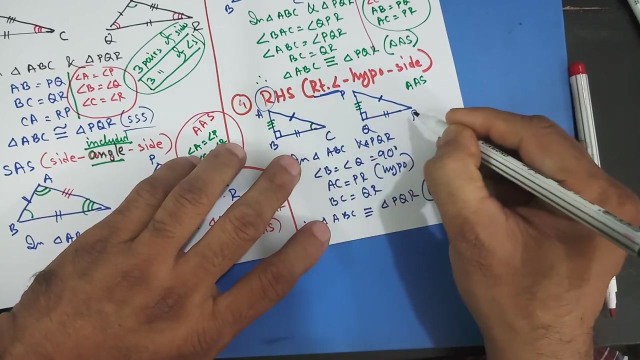 pq, and this ac equal to pr, ac equal to pr. okay, so that's done, and over here i have right angle, one angle, so i can say that other two angles, corresponding angles, are equal to each other. and then two sides are given, so third side has to be equal, so i can say angle c equal to angle r, angle c equal to angle. 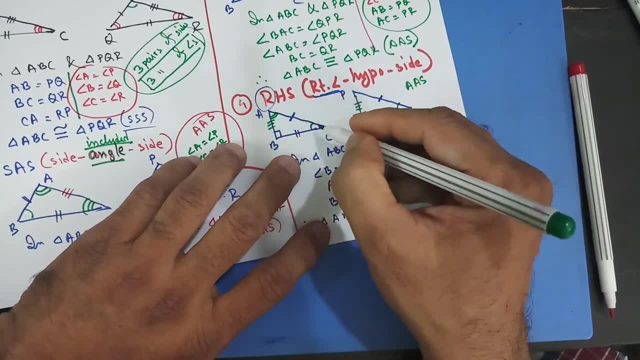 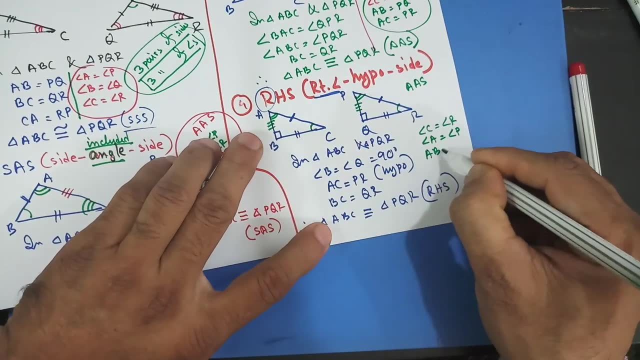 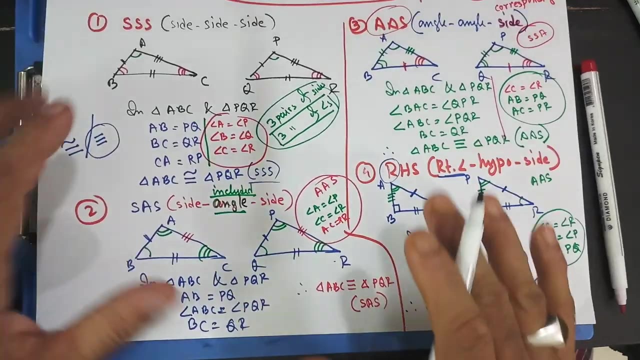 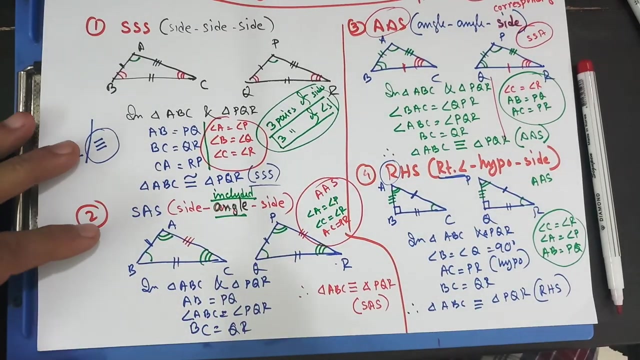 r from these two triangles and angle a equal to angle p, angle a equal to angle p and ab equal to p- q. okay, so that's done. okay, um, i hope you understand the test of congruency for the triangles. uh, in my next video i'll do a test of similarities. okay, thank you for watching. have a.